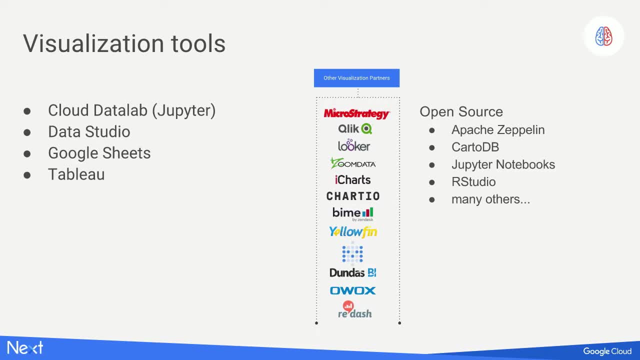 And for the tools that we're going to use. we're going to see a bit of Cloud Data Lab, which is a Python environment for building visualizations and doing some machine learning tasks. We're going to build some dashboards with Data Studio. 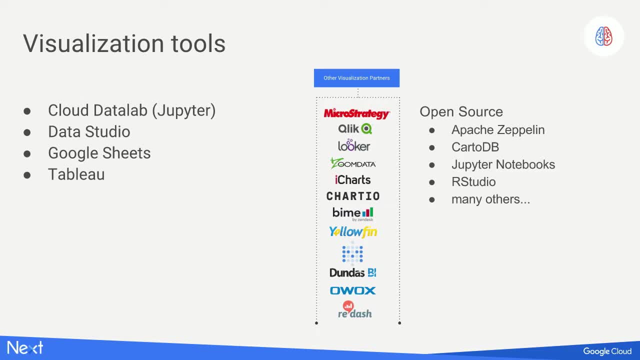 And no visualization talk is complete without talking about spreadsheets. So we're going to use Google Sheets a little bit today, And then Tableau is going to come on stage and demonstrate their powerful visualization tool. Google Cloud connects to many other visualization tools via our partner companies. A few of them are listed here And many open source. 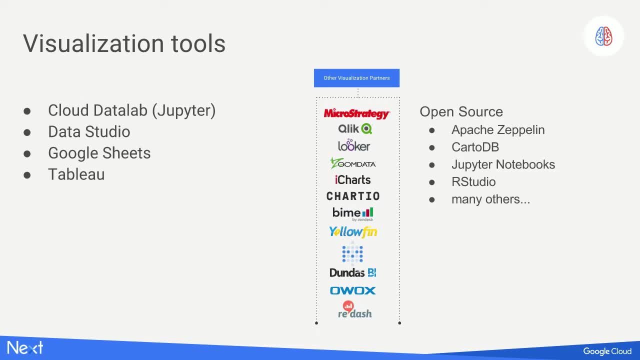 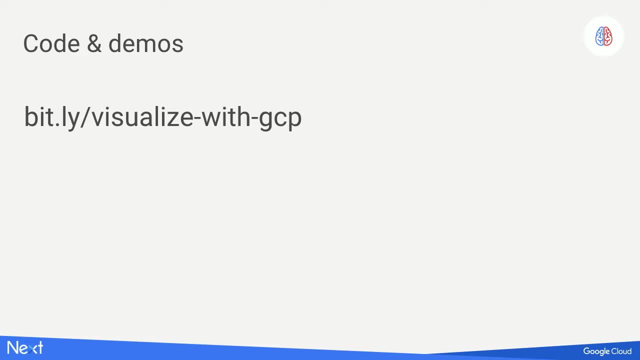 tools let you connect easily to Google Cloud. You're going to see a lot of code today. I don't want you to worry too much about understanding it because I'm going to zip through it pretty fast. I made a blog post here. You can go to that link. bitly visualize. 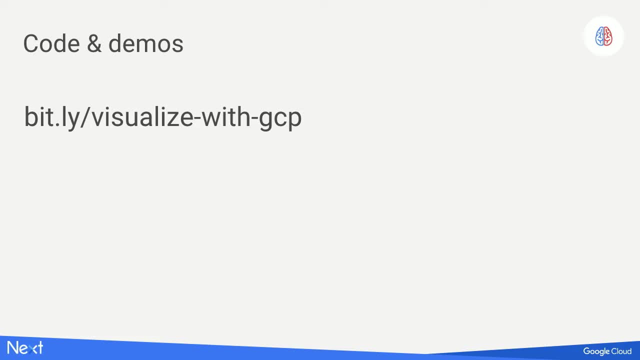 with GCP And I've got links to all the demos I've done with source code. Yeah, Okay, So why are we visualizing our data? The big reason to visualize your data is: you've got a problem you want to solve. 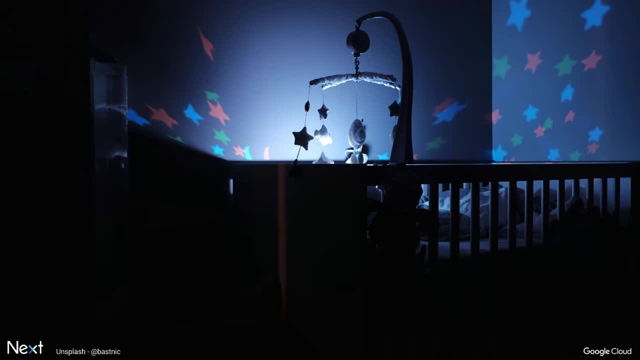 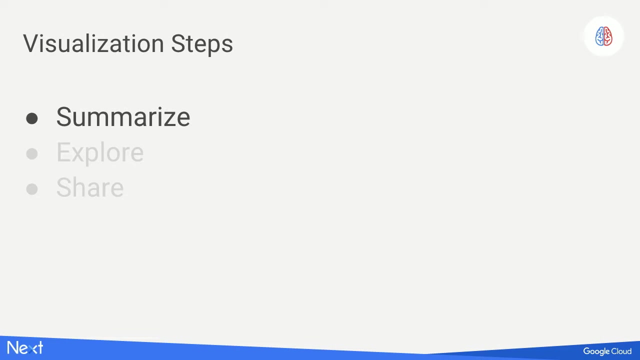 So One problem that a lot of people have is how to name a child. Now, that's a very personal decision, But I'm a geek, so I want to try to use big data to help solve this. The first thing to do when you're building a visualization is to build a summary of the 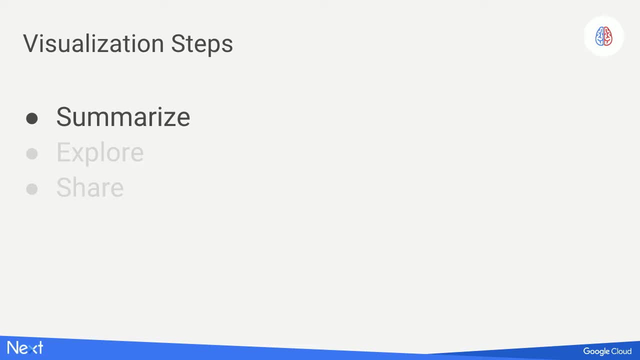 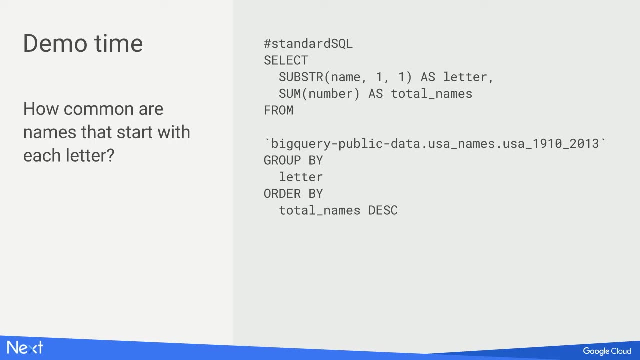 data. It doesn't make sense to try to see gigabytes and gigabytes of data all in one plot. We want to build a nice summary and visualize that. So the way we're going to do that is with BigQuery. So for our name assignment task, we might want to try to. 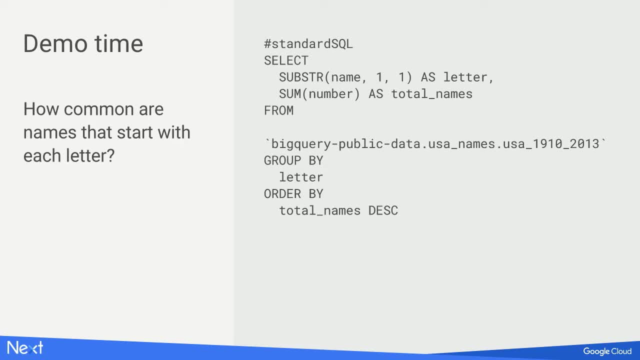 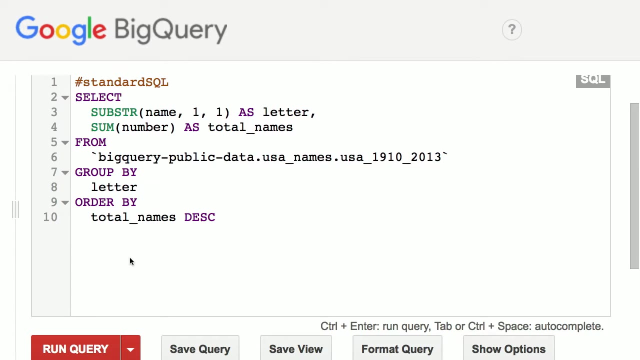 get a feel for what names are out there and how are they distributed. So this query selects the first name, first letter of all the names in the USA names database and counts how many names start with that letter. Now let's cut to the demo. This is that same query, but in the BigQuery UI. I'm going to 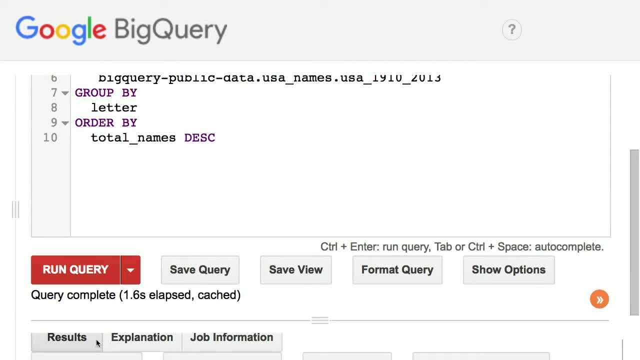 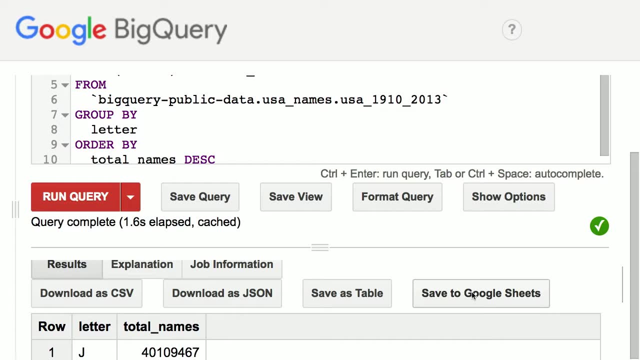 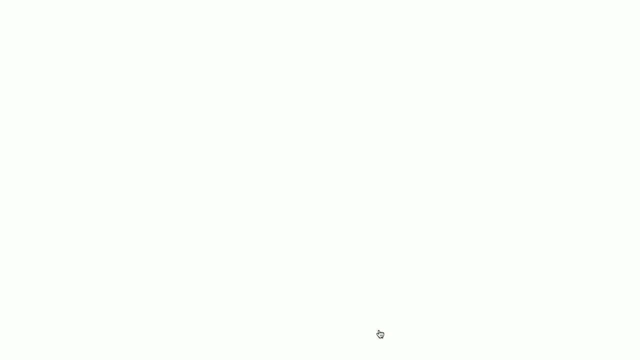 click this red button Here to run the query And that's going to take a few seconds And once that completes, we're going to click this Save to Google Sheets button in the right corner And then we'll click to view that It's opened a new tab And then, once that loads up, we're going to 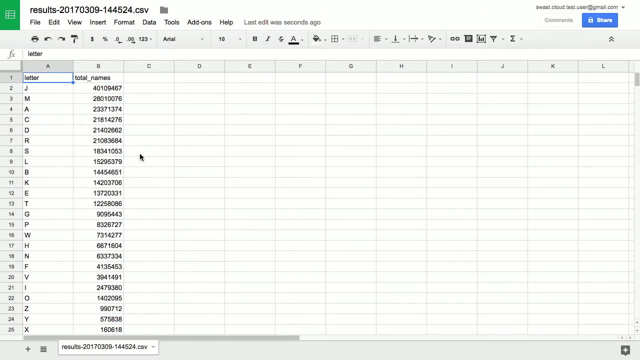 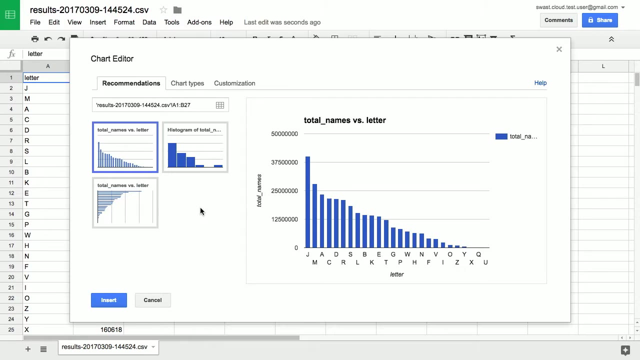 see the results of our query in a Google Sheet. Now I don't care too much about the exact numbers. What I really want is to get a feel for the distribution, So I'm going to insert a new chart Google Sheets recommends, based on the types of data it sees, different visualizations. 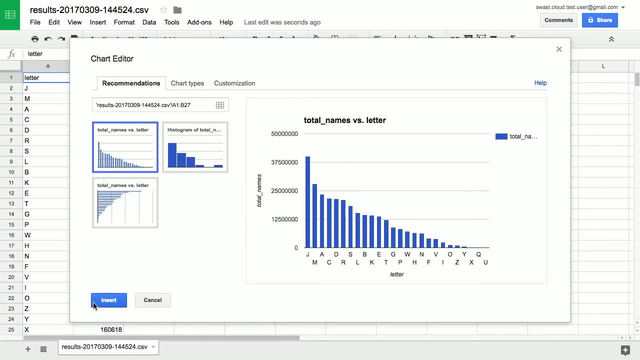 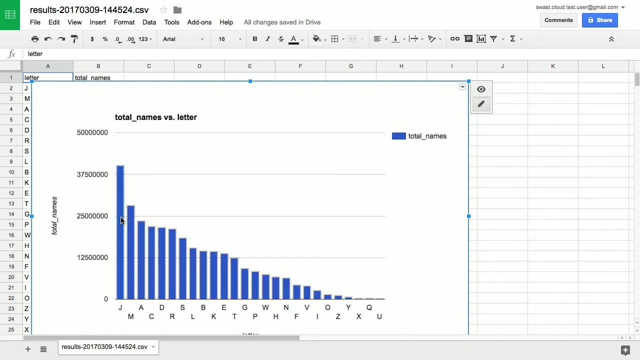 In this case, it's suggesting a bar chart, which is exactly what we want. Let's insert that. So now we can clearly see that the letter J on the left is by far the most popular starting letter for names, And then it trails off slowly, eventually getting down to the letter U, which is so 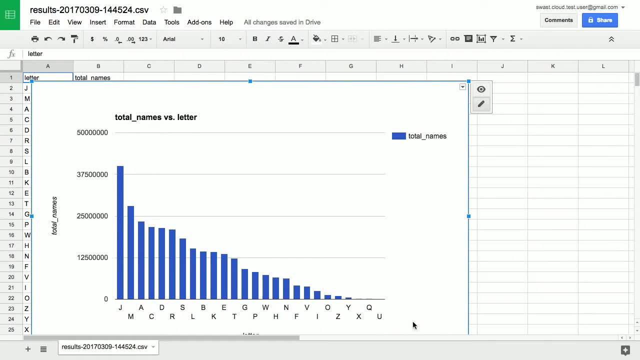 infrequently used. it doesn't even show up as a bar on this bar chart, So maybe, if you're going for a unique name, pick one that starts with the letter U. Ursula or Ulysses might be a good option there. 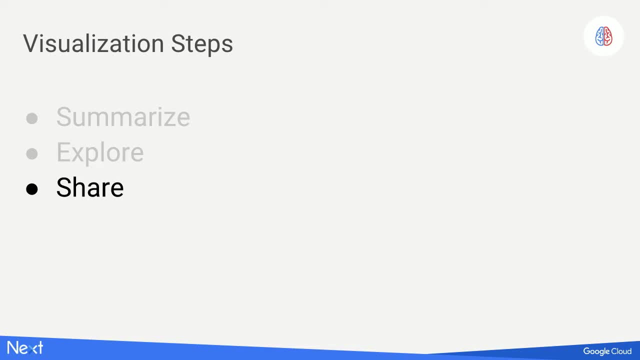 So we've explored our data by building a visualization, And the great thing about Google Sheets is it's easy to share it with your coworkers. So I'm going to click Save to Google Sheets And that's a really good way to share it with your coworkers. 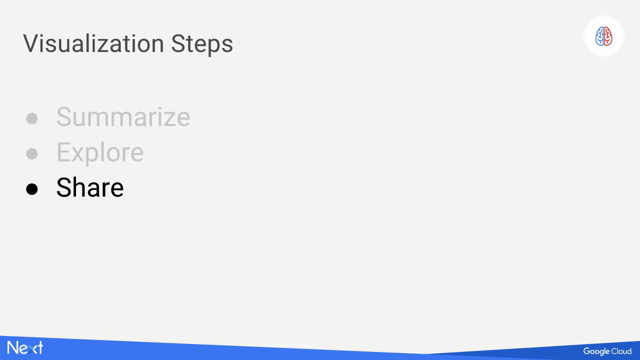 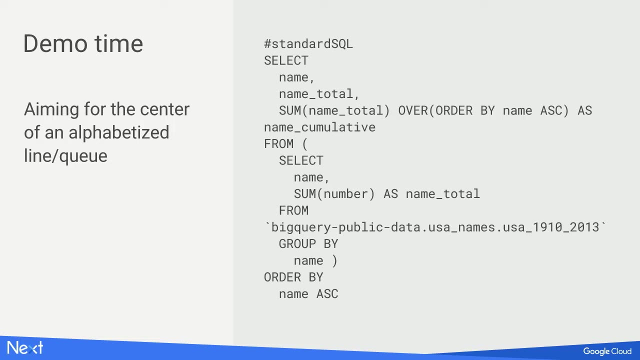 So they can see both the results of the query and the visualizations you've built. Now there's a problem with a potential problem with picking a name that starts with the letter U. I know I experienced this in elementary school. So you're back in elementary school and you're lining up to go outside for recess. 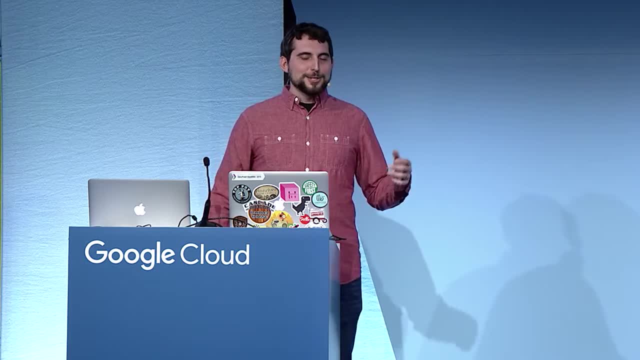 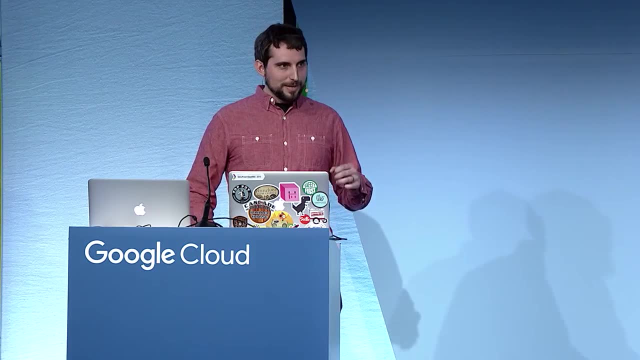 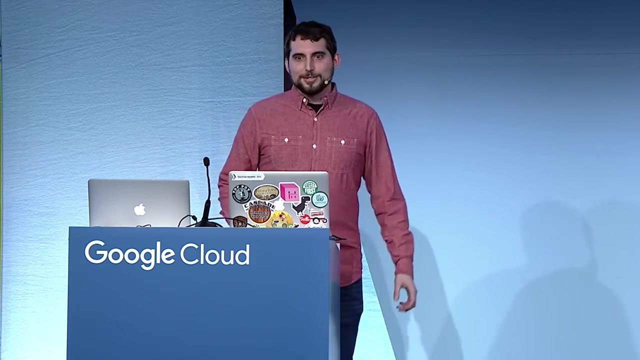 The teacher's going to line you up alphabetically And it's really uncomfortable being at the end of the line of the line, And it's also equally uncomfortable being at the beginning of the line. So I know, growing up I wanted to be in that nice comfortable center spot. 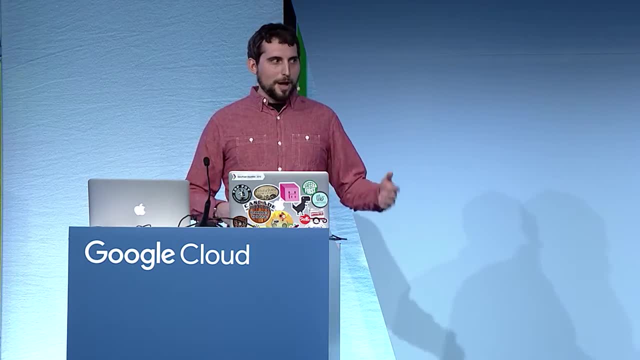 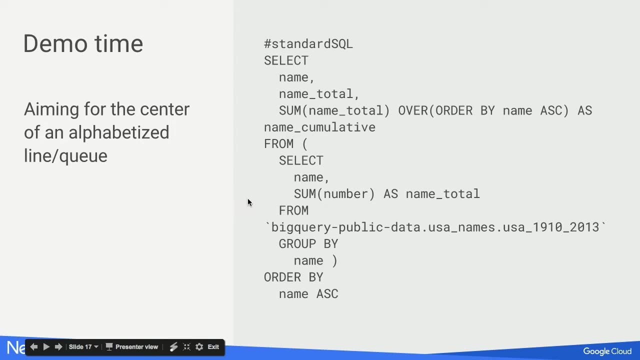 So let's see if we can build a visualization to help optimize for that in our name. So to summarize the data, we're going to run a different SQL query. In this case we're looking at all the names in the dataset and counting how many people. 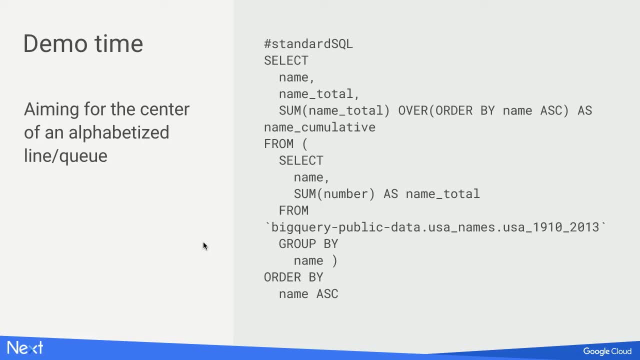 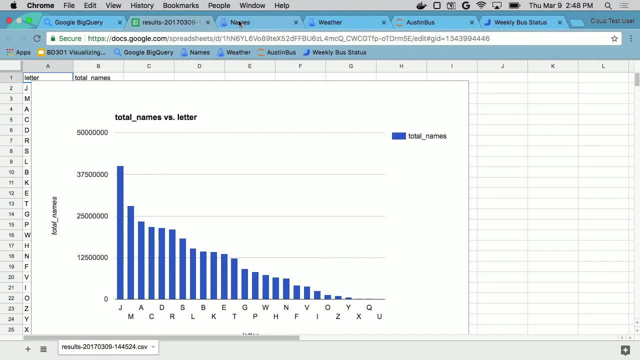 total have had that name. That might seem like a lot of data, and it is, but it's a small enough set that our visualization tools can handle it and it lets us filter it in different ways after we've run our initial query. 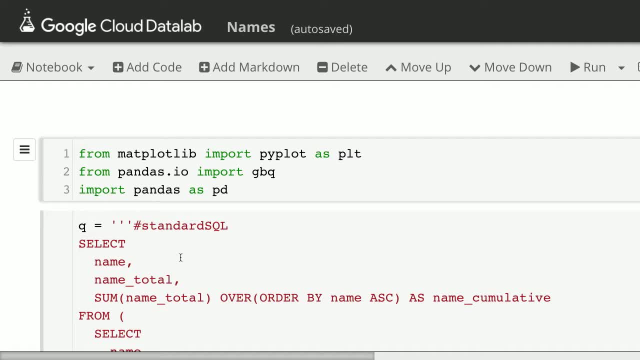 This is Cloud Datalab. It's a Python Jupyter notebook environment And what that means is it's built up of these gray boxes which are called cells. So these cells have Python code in them And you see, they're highlighted in gray right now. 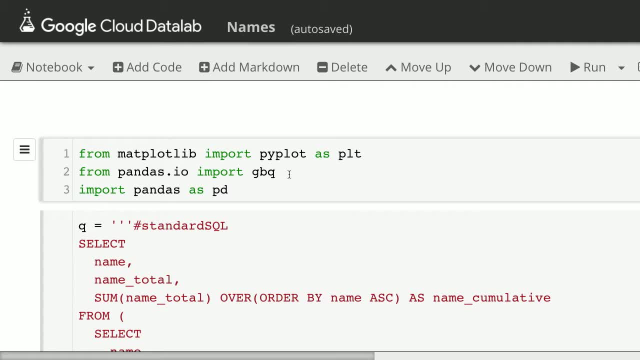 That means I haven't run them yet. So what I'm going to do is I'm going to click through and hit the shift and enter key on my keyboard and that's going to run the code live. So the first thing we're doing is importing some libraries. 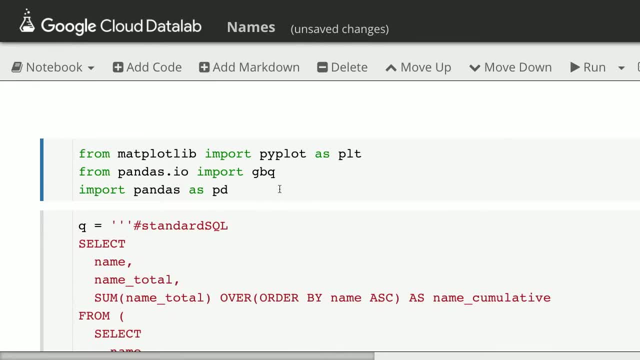 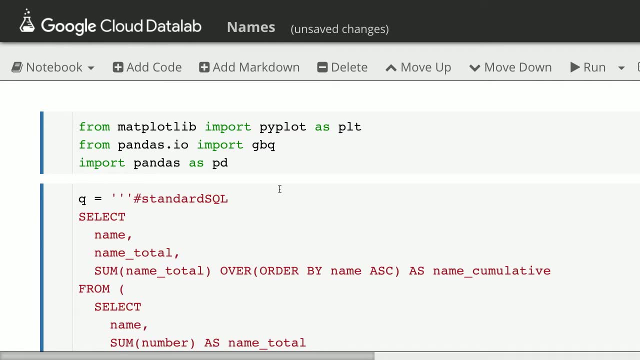 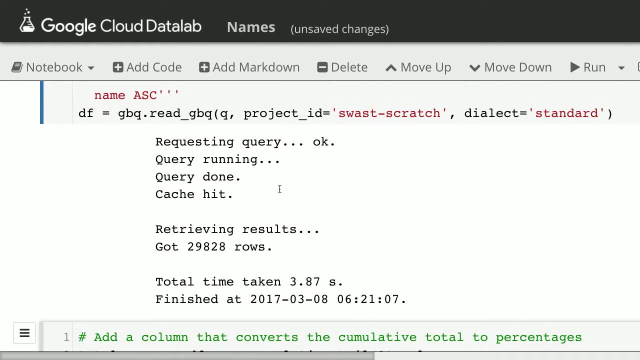 Those libraries might be familiar to many Python programmers. We're just using matplotlib, which is very common for building visualizations in Python, and pandas for doing our analysis and also doing our BigQuery query. So our query completed and you see there's about 30,000 rows here. 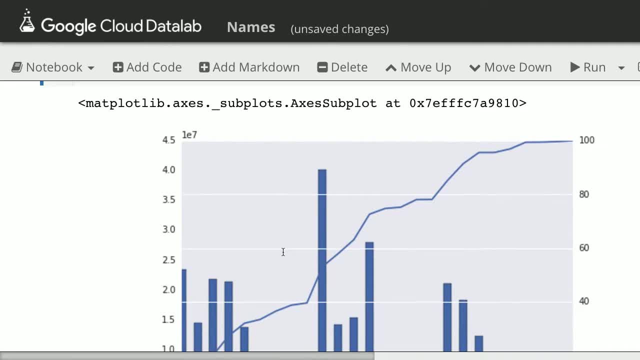 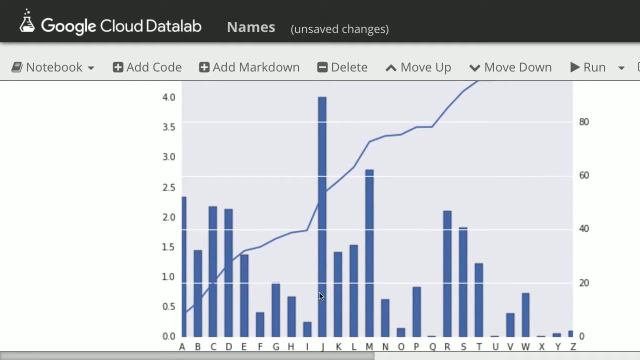 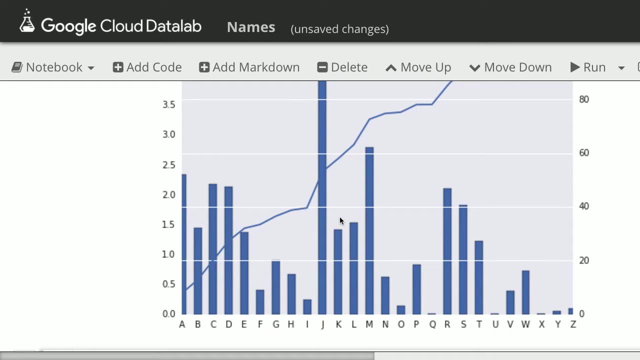 So let's build a chart of that. This is called a Pareto chart. It's basically a bar chart, because you can see the bars here. very much like the previous plot, we saw Extra line graph here, And what that line graph represents is the cumulative total. 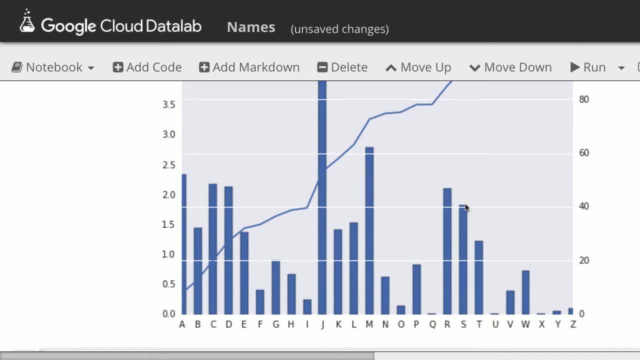 So, for example, at the letter I, you see it crosses the 40% mark. That means 40% of names begin with the letters A through I. So anything at I or appearing before it. Now what we're looking for is that nice center spot. 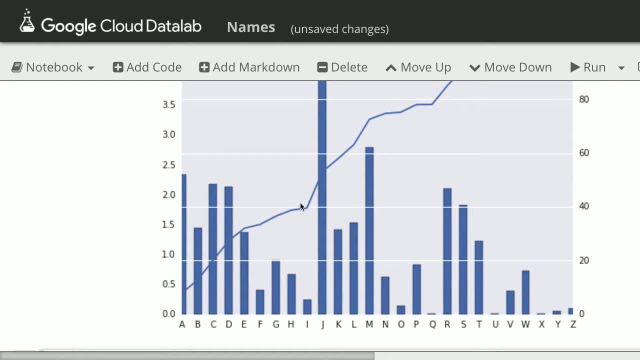 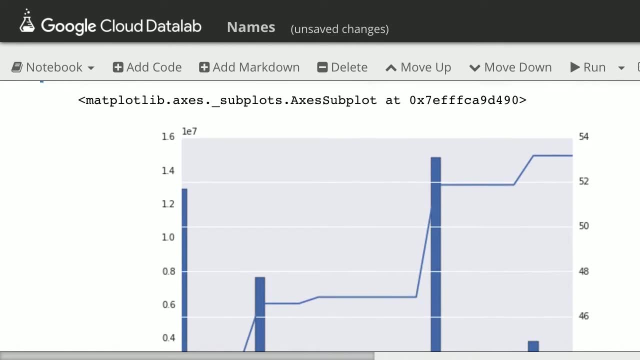 So we're looking for where it crosses the 50% mark, which seems to be at about the letter J. So we're looking for where it crosses the 50% mark, So let's zoom in on that. So here's another Pareto plot, this time with the first two letters of the different names. 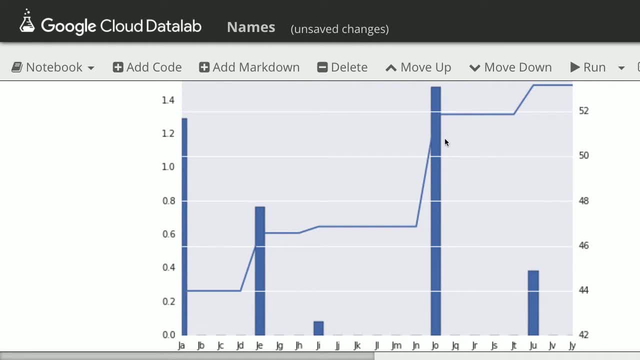 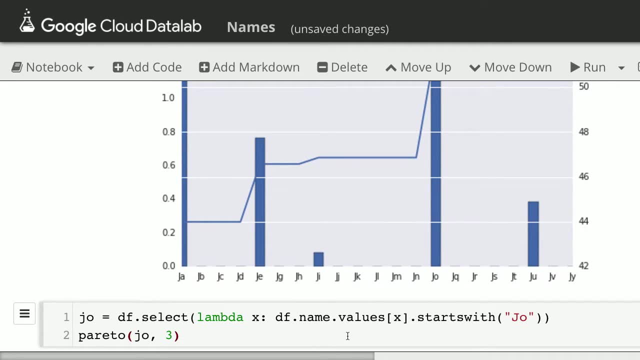 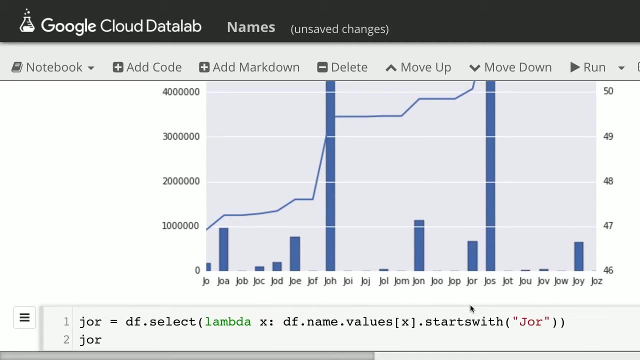 this time starting with the letter J, And we're looking for that 50% mark again. So we've got the letters JO, So maybe start a name that begins with JO. So zoom in again And again, look for that 50% mark line and we see it crosses at JOR. 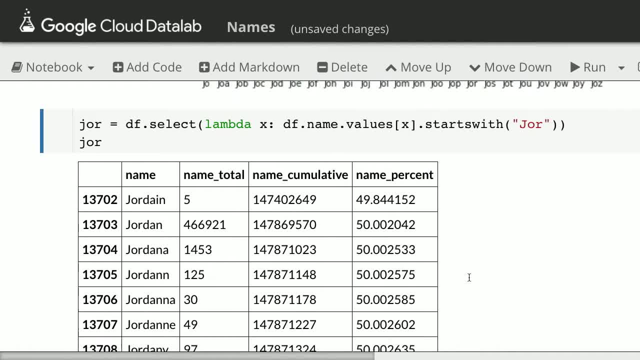 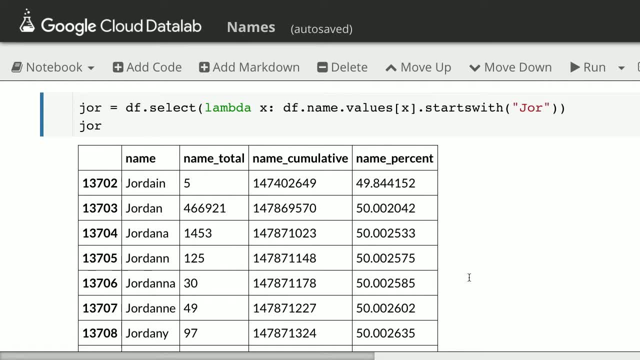 Now for our final visualization. We're actually going to do a table, And a table is technically a visualization, But in this case it is the most appropriate one, because we're looking for a specific name. So we're looking for that exact 50% mark right where it crosses. 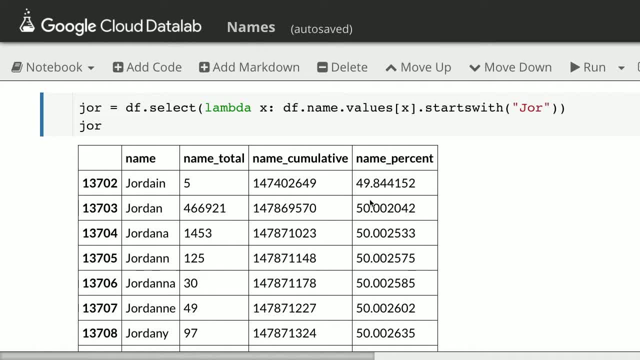 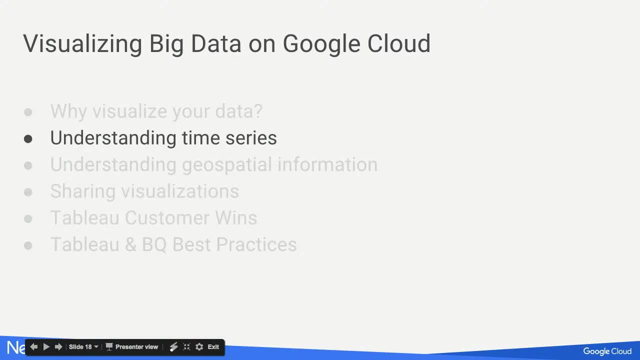 And you see there's some pretty close ties. but Jordan is our perfectly unbiased name. If you pick the name Jordan, you're going to have the best chance of being at the center of those lines, And you also know that the sign is�. 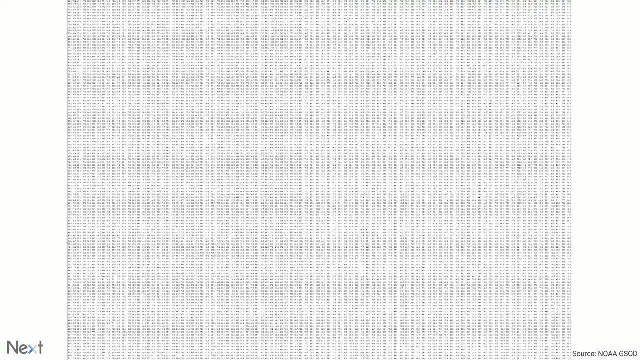 All right, so that was a bit silly, So let's get back to some serious data. This actually does mean something. This represents the last 10 years of weather data from Austin, Texas. So Austin's famous for many things and many festivals, but one of those is the Austin 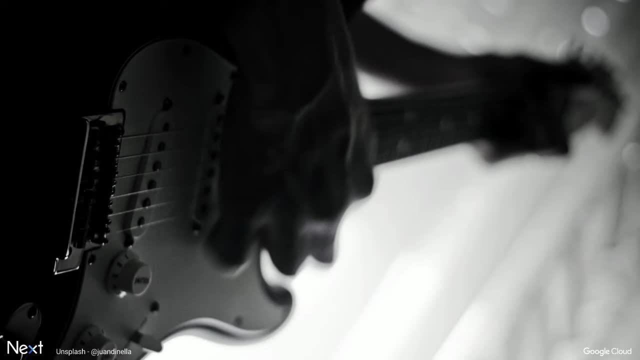 City Limits music festival. So this festival has been going on for over ten years. It's very popular 10 years And a few years ago, back in 2009,, they switched from being on a weekend, primarily in September, to a weekend in October. Now my Austin friends have many theories about. 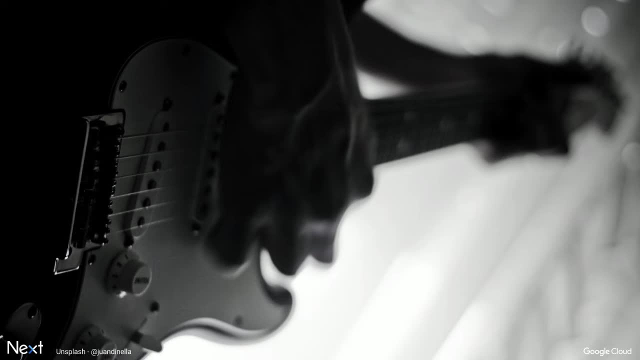 this, but the most common one seems to be: it's really hot in Austin in September, especially for an outdoor music festival where you're out in the sun all day. So my friend's hypothesis is that the organizers switched to October to beat the heat. Now, that's a great theory. 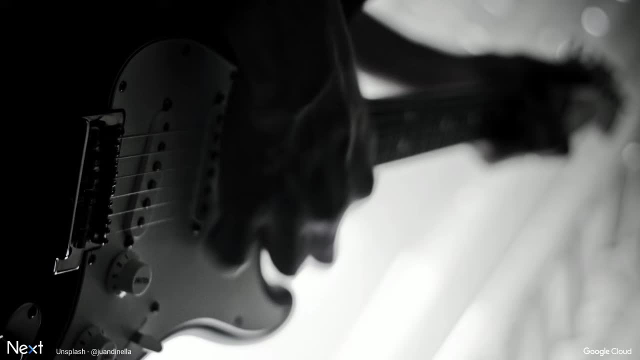 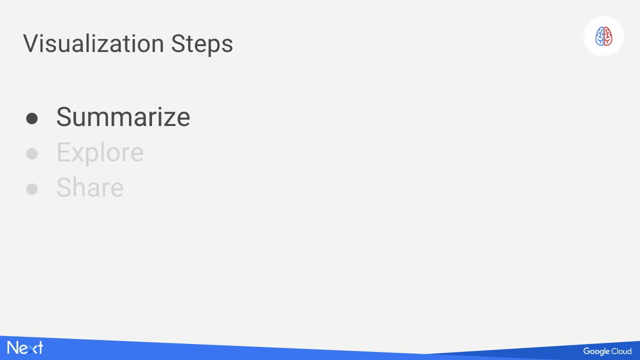 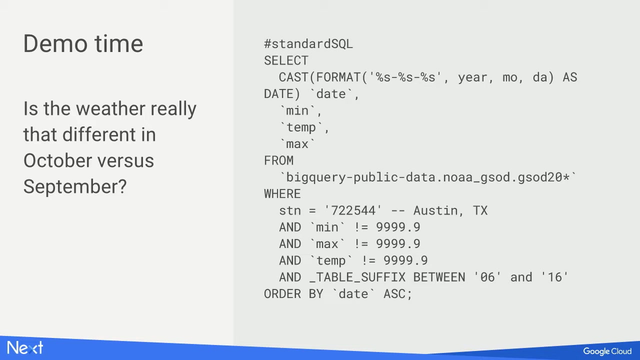 and it seems to make some intuitive sense. but let's use some big data and see if this hypothesis is correct. First thing we're going to do is build a summary, so we're going to run another BigQuery query. This query selects data from the NOAA weather public data set. 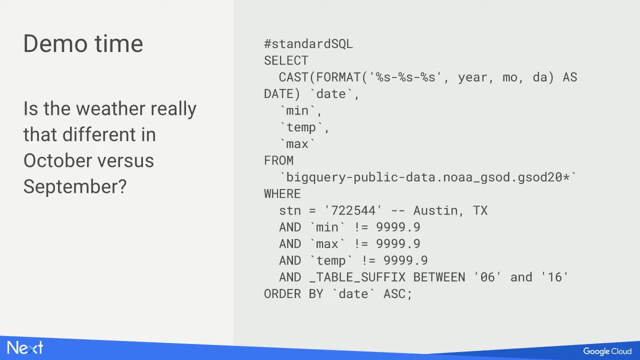 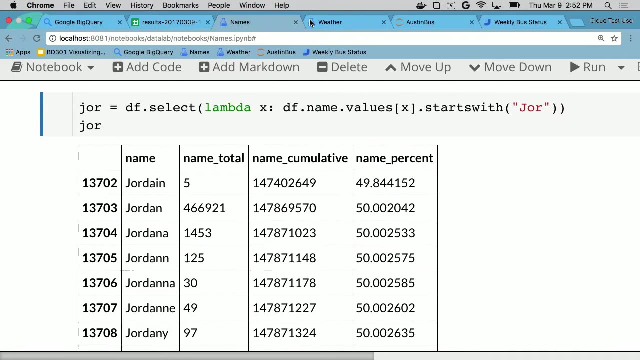 So that data set is over 100 years of temperature data. So the way we're going to filter it down is just select the Austin Texas weather station and limit to just the past 10 years of weather data. Again, we're going to use a data lab. 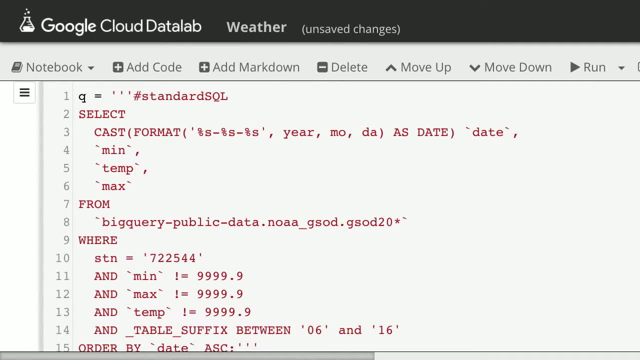 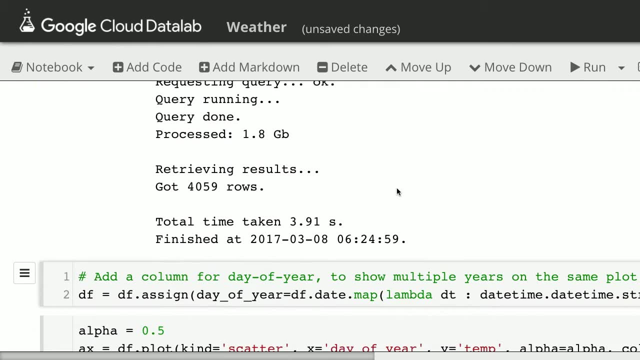 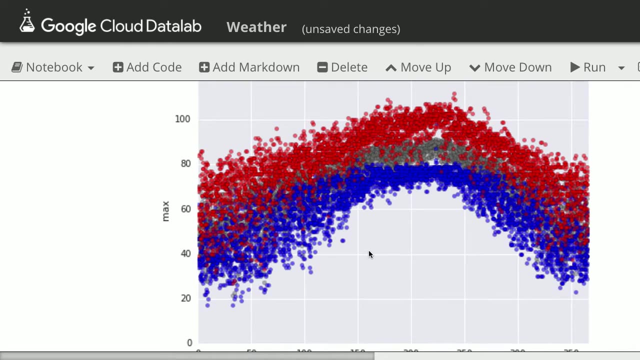 notebook and the same libraries- pandas and matplotlib- And this query might take a little bit longer because it's a slightly larger data set, but it's still pretty fast. Now let's plot this data out. So now this is the exact same set of data that you saw in that slide, but it should. 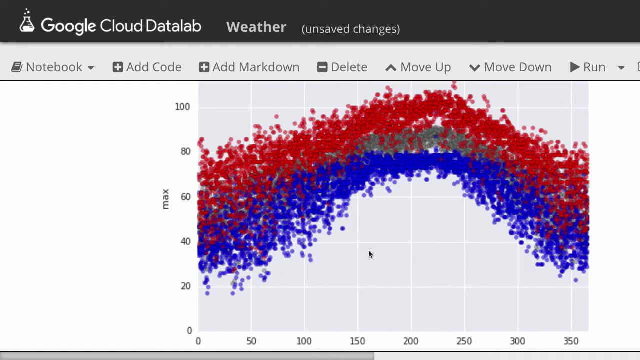 be a lot clearer, the patterns here. So I've taken 10 years of data and then I've overlaid them on top of each other so that you can see the seasonal changes. So the x-axis here is the day of the year and the y-axis is the temperature in Fahrenheit And red means. 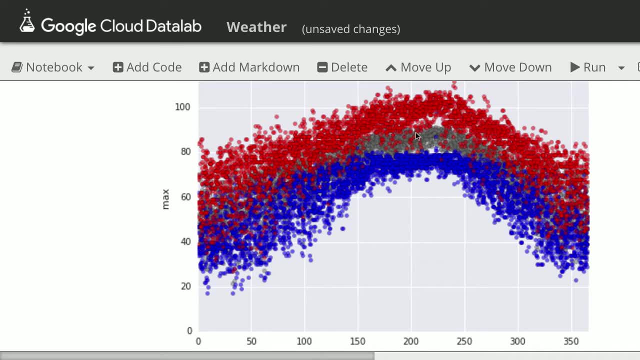 the high temperature for the day, blue is the low temperature and gray is the average temperature for the day. So one thing you can definitely see here is it's a lot hotter in summer as we'd expect, and actually the variance between temperatures is a lot lower in the summer months versus 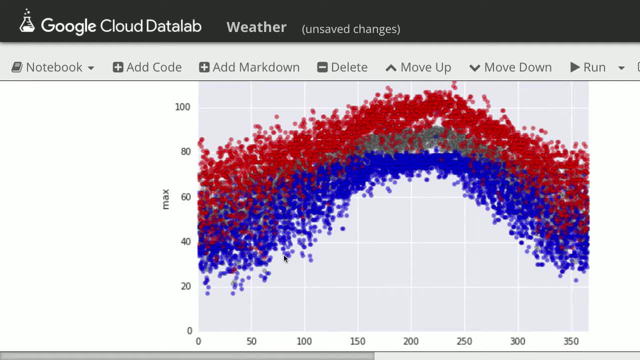 the winter months. They really change throughout the days in the winter. But this graph doesn't answer our question. What we want to know is where our music festivals lie on this line. Let's see that I've zoomed in a little bit. 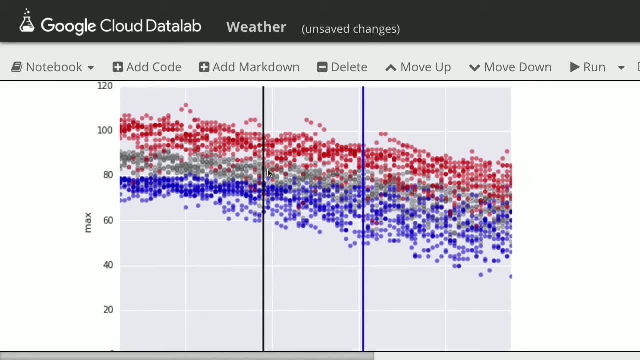 On the left is one of the music festival weekends that happened in September and on the right, the blue line, is one of the music festivals that happened in October. So we can definitely see a downward trend here. There's about five degrees difference. 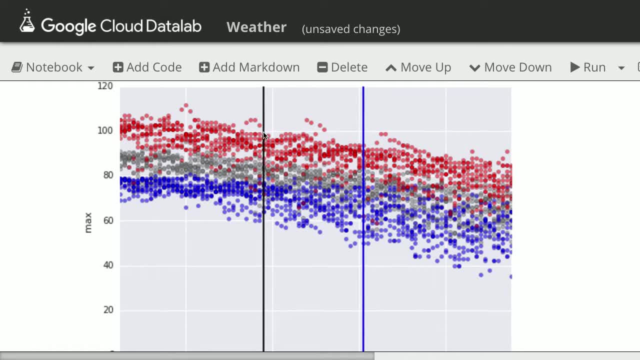 between October and September in the high temperatures and low temperatures, But five degrees is not a big difference, So maybe that's not the primary reason the organization picked October as the month. One thing about choosing October is the first year that the Austin City Limits Music Festival. 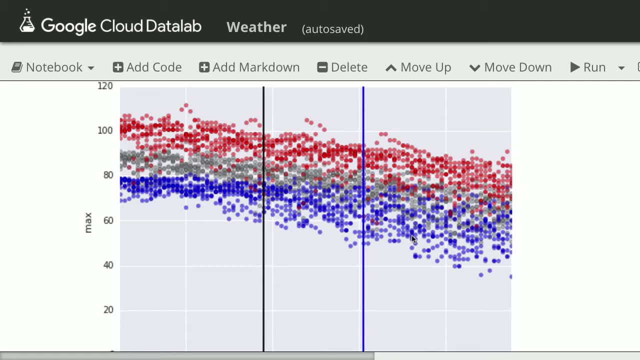 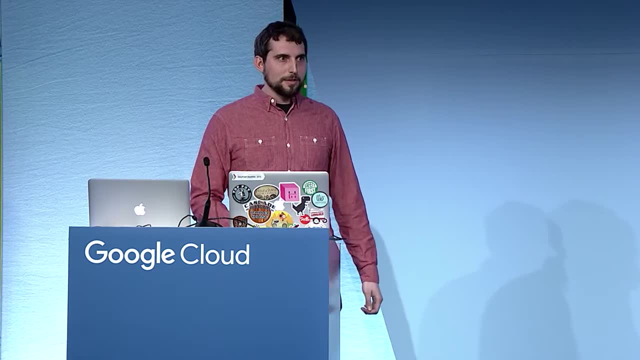 was in October. there were torrential downpours all weekend, So this outdoor music festival was a really muddy mess, and they had spread compost out on the lawn before, and so it smelled really bad too. So maybe, if you're picking an ideal weekend, you're going to want to make sure that you 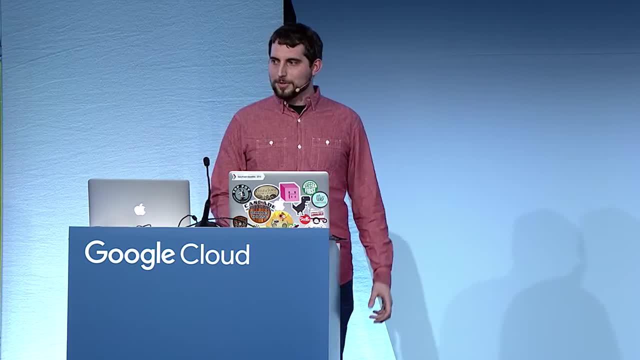 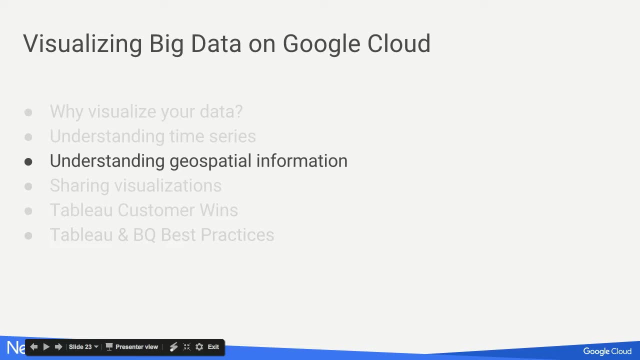 pick an ideal weekend based on the weather for your outdoor music festival. Maybe pick it on more than just the temperature data. So, speaking of Austin, I used to live there for about five years or so And one of the problems I encountered, and wish I had a visualization to help me solve, was choosing where to live. 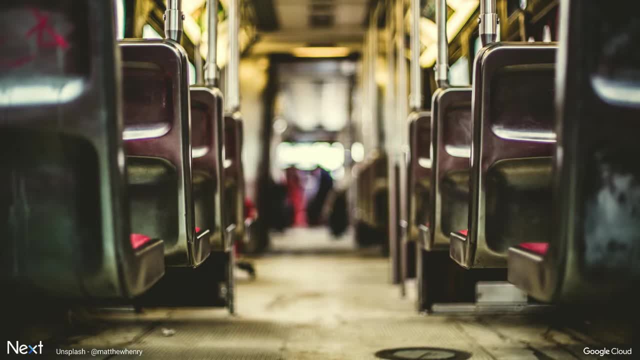 I'm a big public transit nerd. I like to take the bus and the light rail whenever I can – even in Austin, where it's 100 degrees out and I'm outside in the hot sun, I'll still take the bus. So maybe my ideal spot would be close to a reliable public transit station. 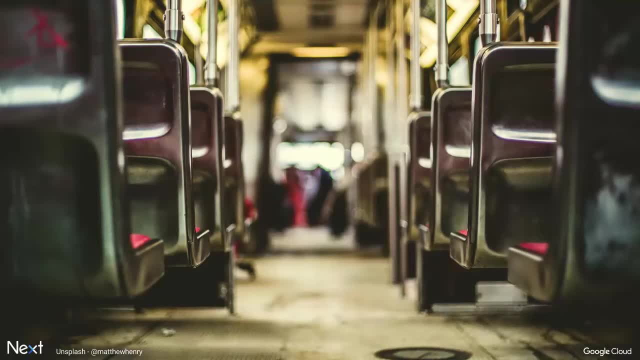 The other thing about living in Austin is you learn to love the taco. You end up eating tacos every meal of the day, but especially breakfast. My ideal spot would be somewhere that's both close to reliable transit, but also close to some of my favorite taco shops. My ideal spot would be somewhere that's both close to reliable transit, but also close to some of my favorite taco shops. 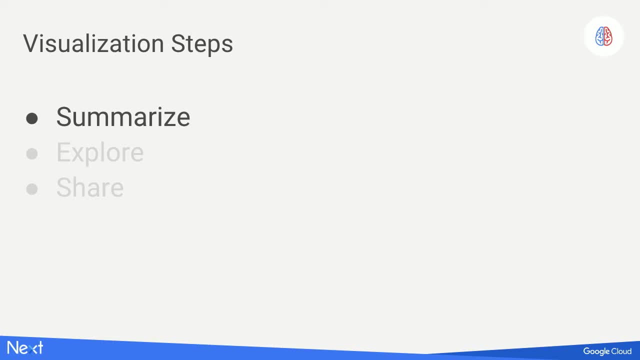 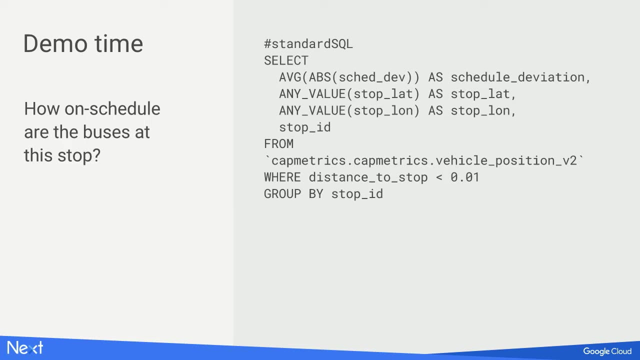 My ideal spot would be somewhere that's both close to reliable transit, but also close to some of my favorite taco shops. So let's build a visualization to help us solve this problem. We're going to summarize the data again, again, with BigQuery. This time, we're going to query a data set called. 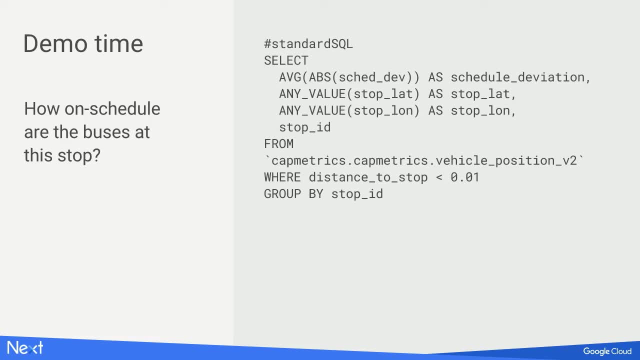 CapMetrics, which was uploaded by a member of the open data community, Sean Cascetta, to a public BigQuery data set, And this data includes bus tracking data, so times and locations of all the buses, As well as the bus stops. So what I'm selecting here is whenever a bus is at a bus stop. I 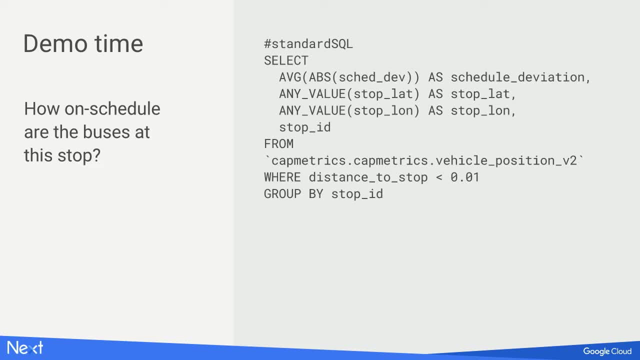 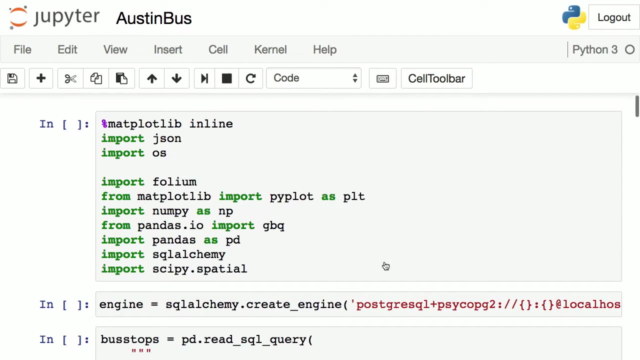 want to know: is that bus on schedule or off schedule? Because I'm using that as my measure of how reliable the buses are. I'd rather the bus be on schedule than off schedule. So back to the demo. This is another notebook and this is more Python code here I'm using 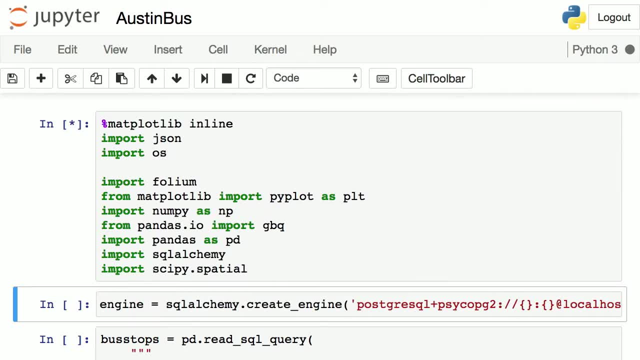 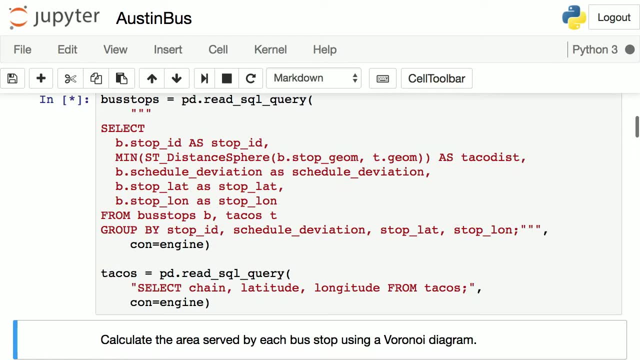 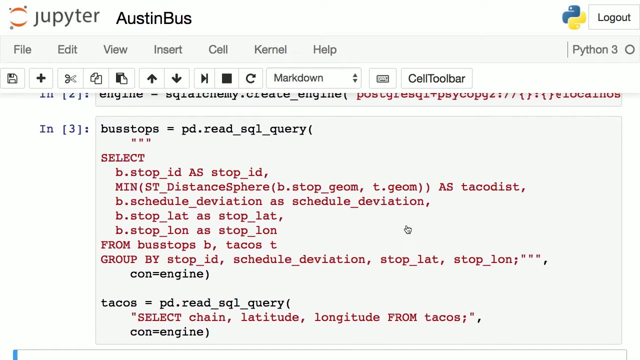 pandas and matplotlib, but a few other libraries here to work with geographic data, and also I uploaded the query results to a Cloud SQL Postgres instance. The reason I did that is because the Postgres instance supports the post GIS extension, which allows me to do GIS queries against it. 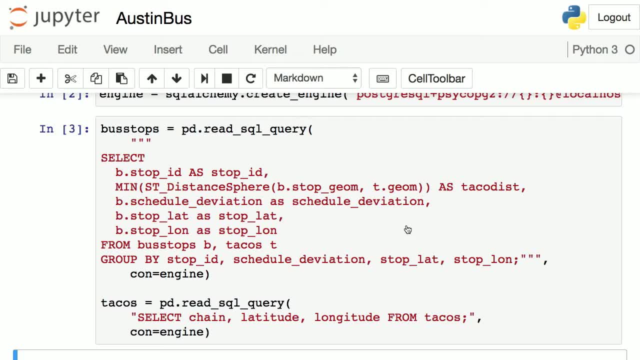 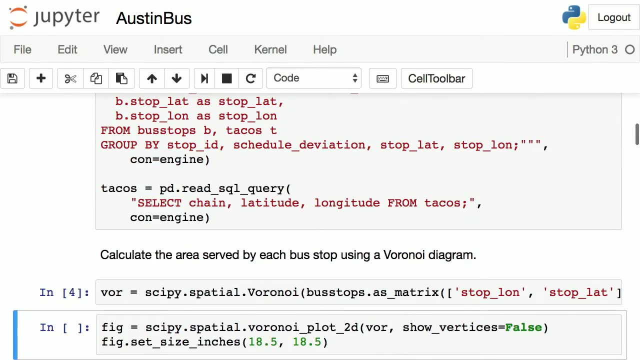 In this case, I've got my bus tracking data and I also added a table for my favorite taco shops, So I'm selecting the distance to the closest taco shop via SQL. All right, so the query's finished. Let's build a plot of this. 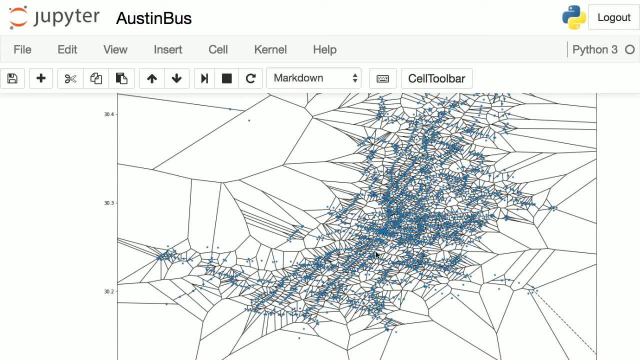 This is called a Voroni diagram. It gives you an idea of where the bus stops are. that's these blue dots here, but also the area of the bus stop. So I've got my bus tracking data and I also added a table for my favorite taco shops. 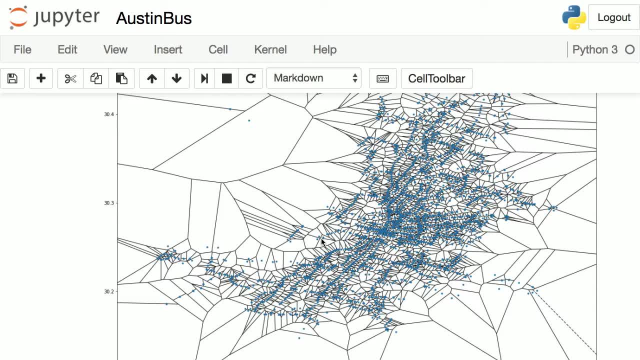 So I'm selecting the distance to the closest taco shop via SQL. This is the area served by that bus stop. These blue dots are surrounded each by a polygon. That polygon, any point within that area, the nearest bus stop is the blue circle contained. 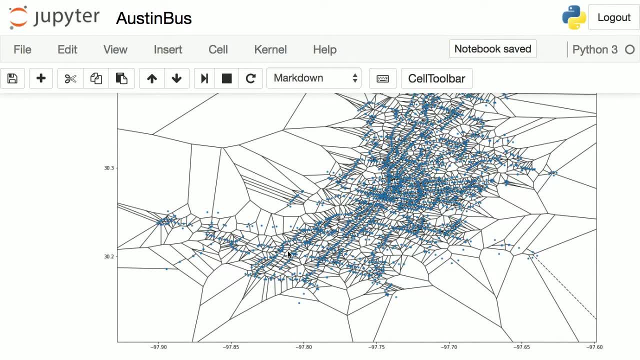 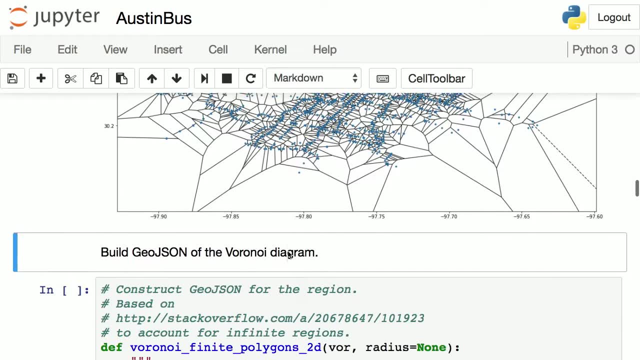 within it. Now I've plotted this latitude- longitude data on just a regular XY plane, and that's not quite the right thing to do, so let's plot it out on a map instead. So I'm going to convert this Voroni diagram into a GeoJSON. 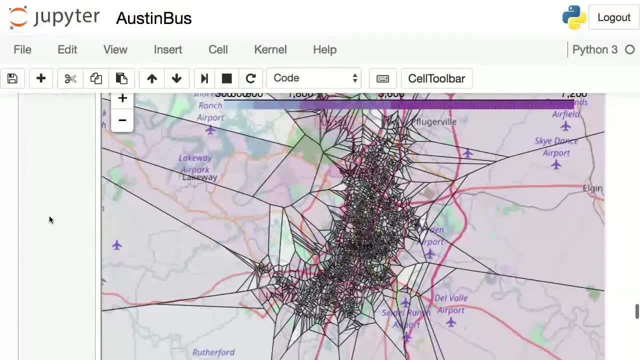 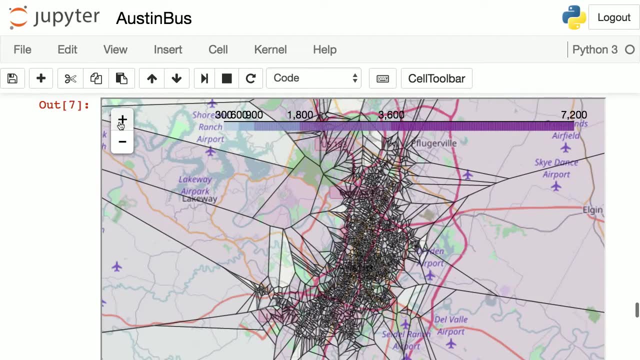 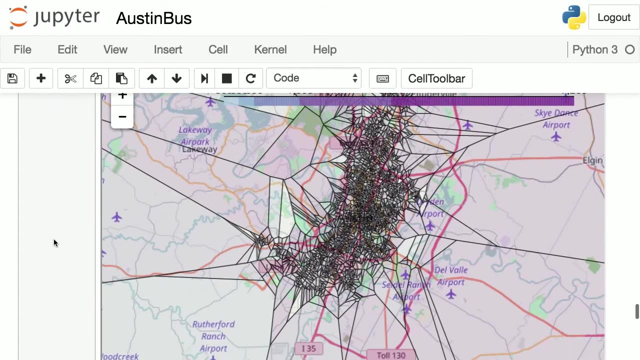 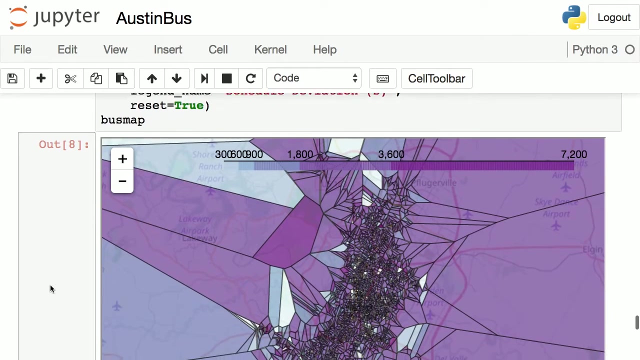 And then I'm going to plot it out using a library called Leaflet. So here's all our bus stop areas plotted out on a map, So you can see the different areas served by the bus stops overlaid on the map of Austin. This doesn't quite answer our question, so let me color it in, based on the reliability. 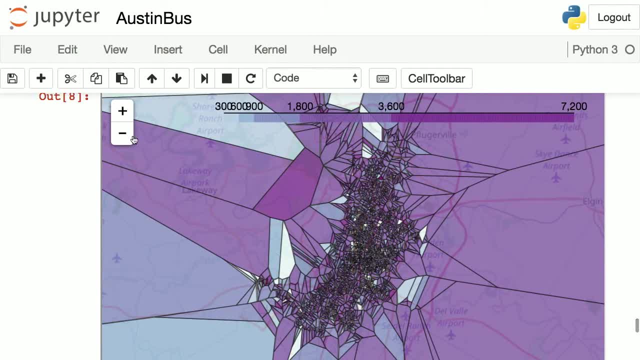 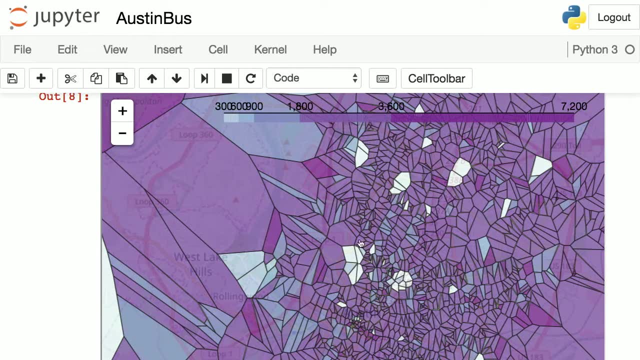 of the buses in those stations. So now we can see the dark purple areas. These are where the buses are not so reliable. They're off schedule on average by quite a bit. And the lighter areas are where the public transit is pretty reliable and they're on. 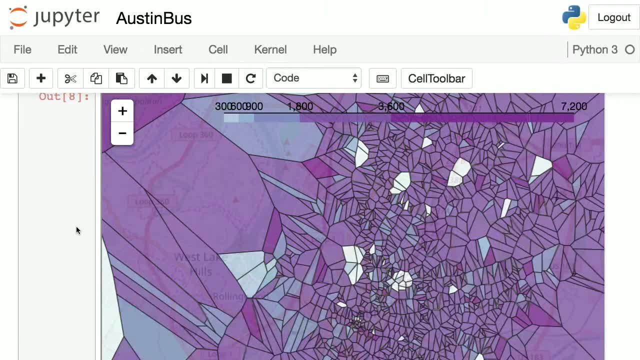 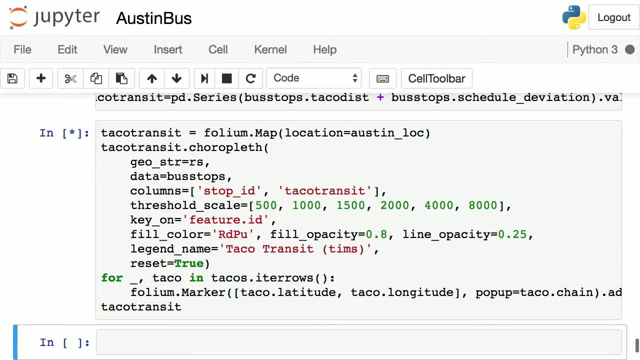 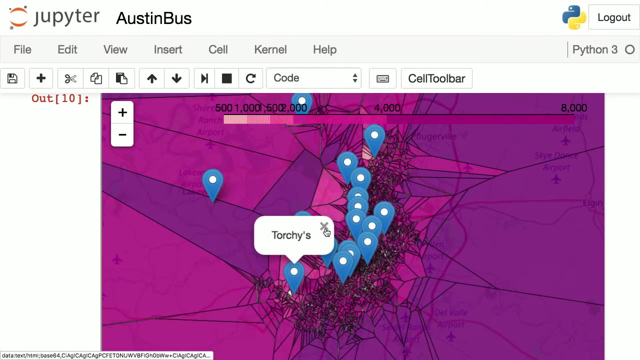 schedule most of the time. So that's great, We could use this to find an apartment, but it doesn't solve my taco problem. So let's combine the taco table with this data set. So now I've overlaid. I've overlaid where all my favorite taco shops are. 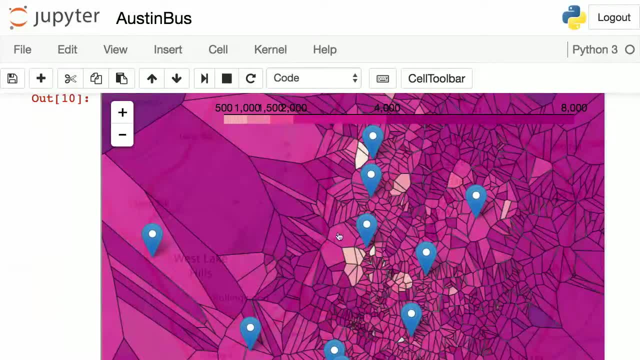 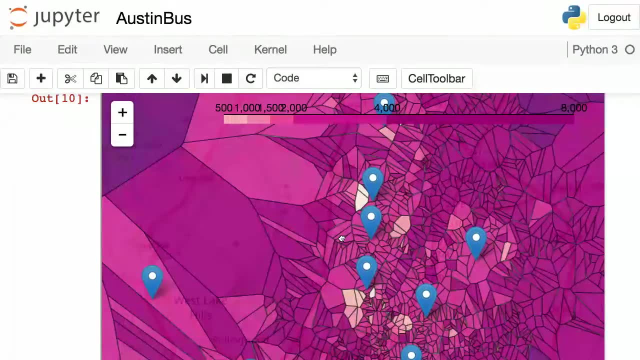 And then I've colored it in not only by the public transit reliability but also the proximity to a taco shop. So the light areas are the areas that have reliable transit and are close to a taco shop, And the darker areas are either not reliable or far away from a taco shop, or both. 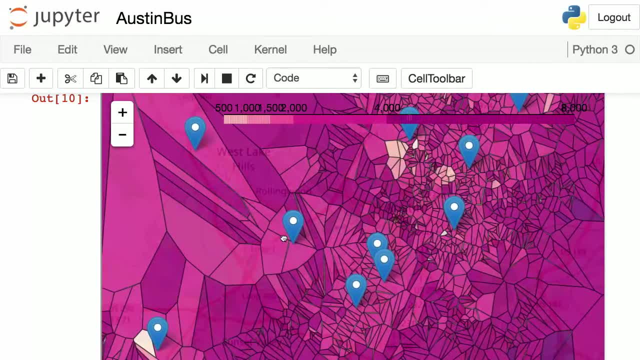 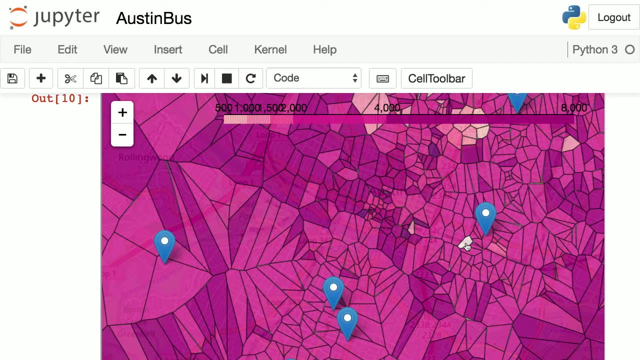 So, panning around, We can see a few possible choices. If we want to live on the south side- I happen to know this is William Cannon Road down here and it's by Torchy's Tacos- If we want to live on the east side, there's not too many choices, but we've got a little. 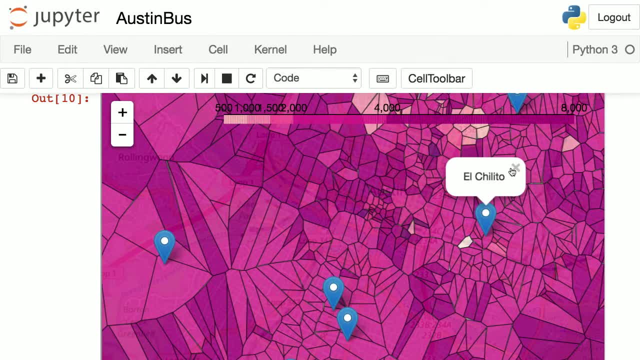 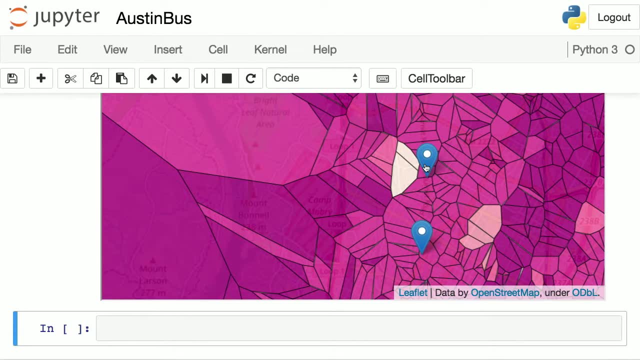 spot of white here by the Plaza, Saltillo Light Rail Station and El Cholito. Or, if we want to live on the north side, there's a nice spot up here across Torchy's Tacos on Burnet Road. All right. 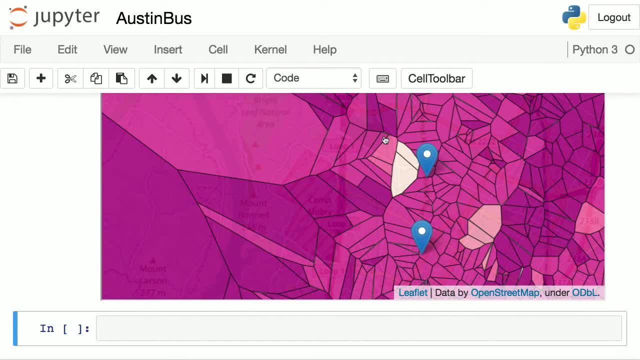 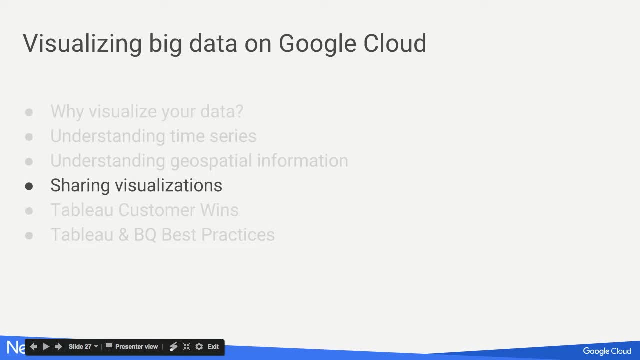 So we found the perfect place to live. It's got reliable public transit and proximity to delicious tacos. So let's imagine for a minute that you're a data scientist and you're working for the public transit company. So you just saw my talk and you want to cut down on the number of those purple areas. 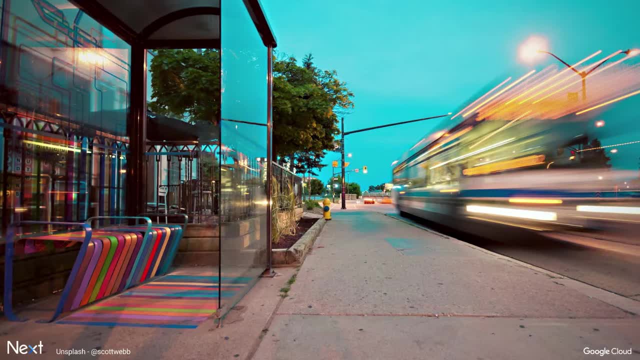 So it's your job to help keep these buses running on time. So you're going to do the same kinds of analysis that we just saw, but eventually you're going to want to share your work with one of your coworkers, So one way to do that is to take a screenshot of your visualization and then send it off. 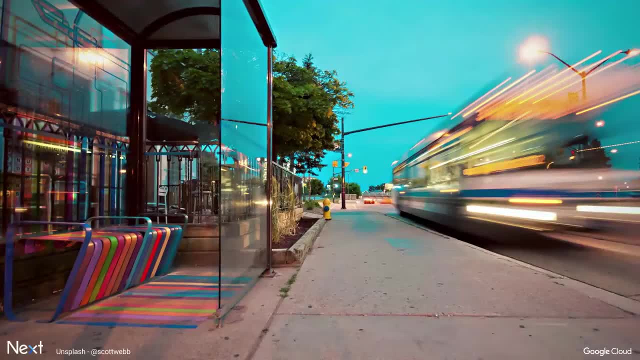 in an email to your coworker. Now that works fine. They're going to see the exact same image you saw, but there's a problem with that. Buses move around, So by the time your coworker gets to that email an hour later, the problem will have. 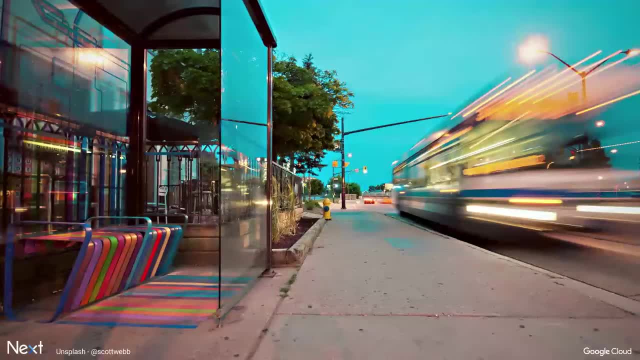 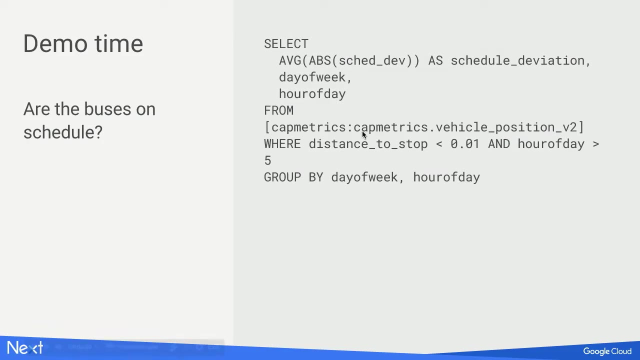 evolved. So ideally, we'd have a live dashboard that shows not the data an hour ago, but the data as it is right now, And we're going to use Data Studio to build a dashboard like that. Data Studio allows you to connect to BigQuery, as we've seen in the other visualizations. 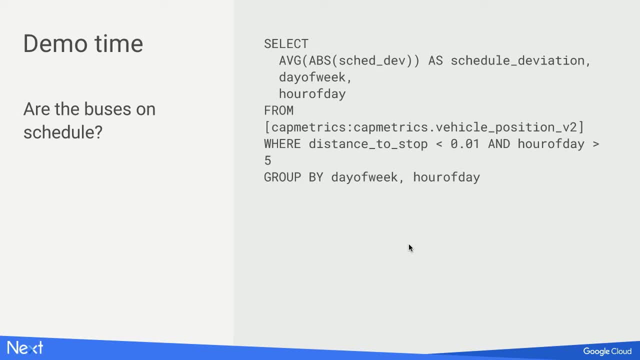 in this talk, But it also supports Google Analytics and many other data sources. In this case, we're going to use a BigQuery query, So this query is very similar to the previous one we saw. I'm still looking at how far off schedule the buses are on average, but this time I'm 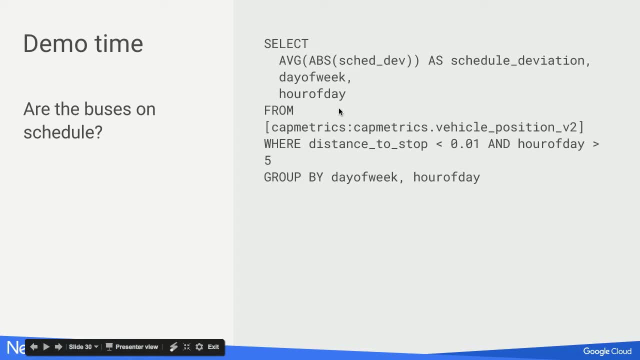 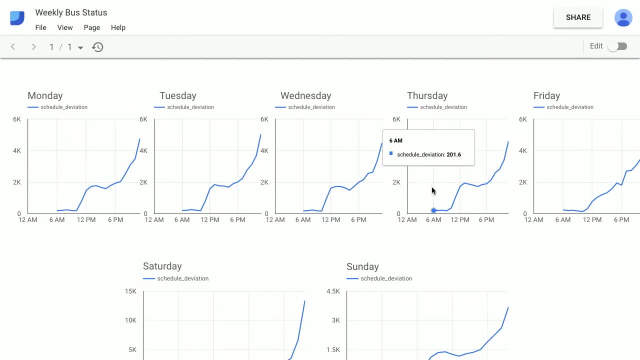 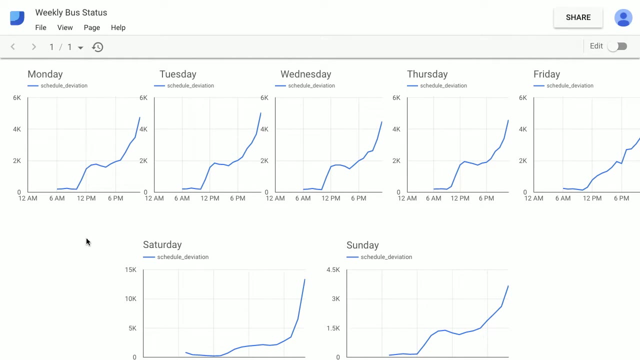 splitting up by the day of the week and the hour of the day because I want to see how the problem changes over time. Cutting to the demo, I built this Data Studio dashboard, So I used Data Studio's filtering mechanism to build seven different graphs. I'm going to show you how to do that. So I'm going to show you how to do that. So I'm going to show you how to do that. So I'm going to show you how to build seven different graphs here, each showing a different. 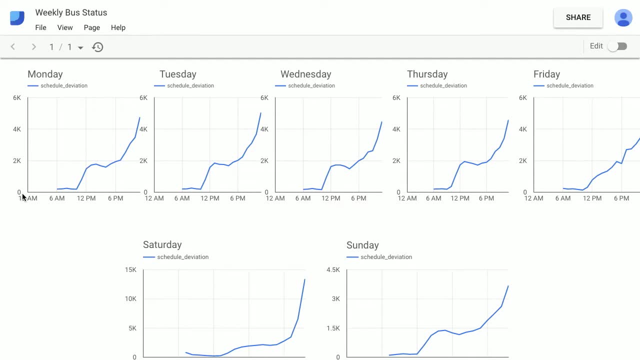 day of the week, And then I've got a line graph for each one. The x-axis is the time of the day and the y-axis is how far off schedule are the buses on average for that hour, So you can see the buses start off on time, which makes sense. 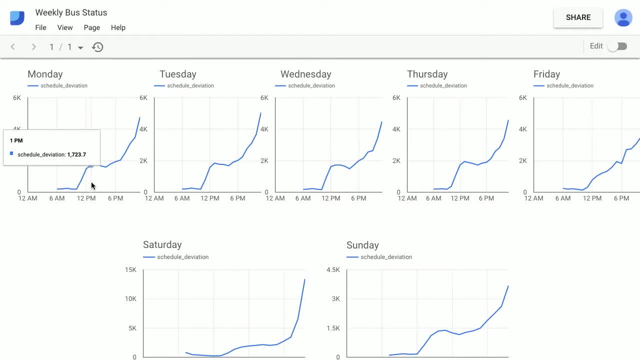 They've just started their route And then they get more and more off schedule throughout the day. In the afternoon they catch up a little bit, but then rush hour hits and they get way out of whack. So the great thing about Data Studio. 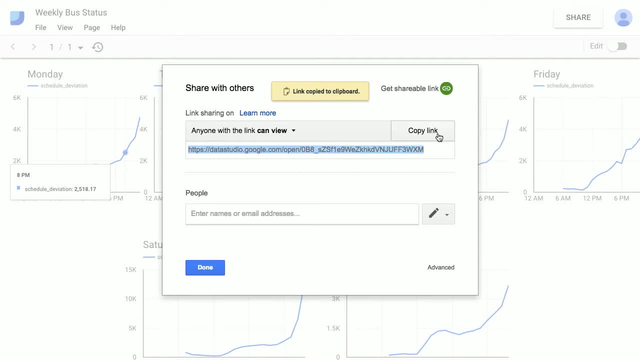 is this share button up here. You can click that. It gives you a link. You can send that off to your coworker And then when they load this page up, it's going to rerun that query and they'll see. 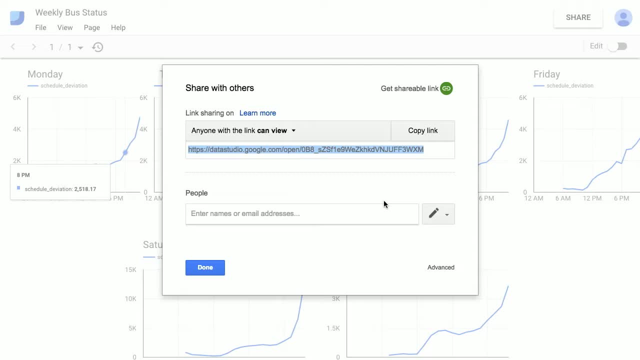 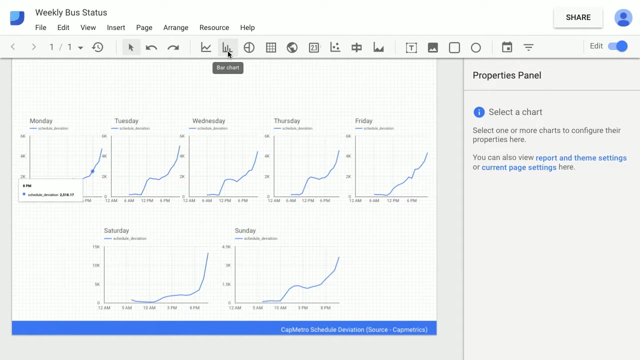 a live view of the data And if you want their help building this dashboard- maybe you want them to add some new visualizations to it- you can give them edit access, just like you would at Google Doc. Now, I've only used line graphs in this dashboard, but Data Studio also supports bar charts. 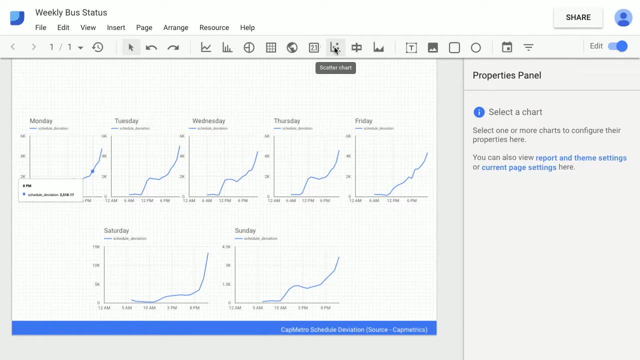 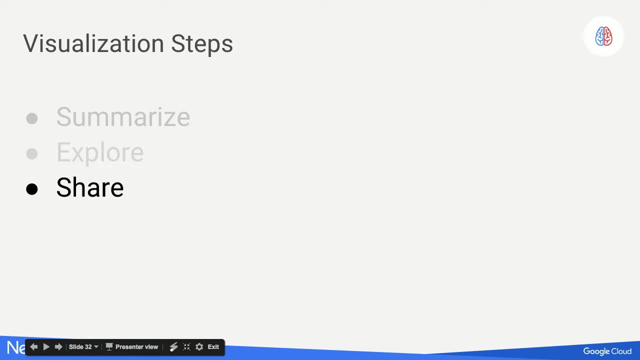 graphic maps, scatter charts, all the visualizations we saw today and more. Data Studio is great for this sharing use case. It's not the tool I'd use for the analysis part, the exploration phase, figuring out what transformations I want to make to the data and how I want to visualize it. 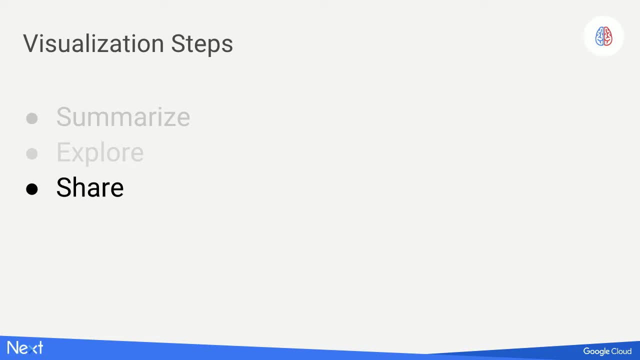 For that I like to use those notebooks. It's really handy to be able to run some Python code. You can use Python code to grab some data, filter it in a bunch of ways and try out different visualizations. So, speaking of code, again, here's the link to the blog post in case you forgot it, and 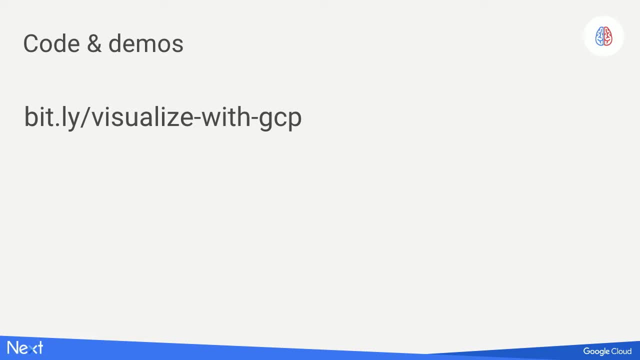 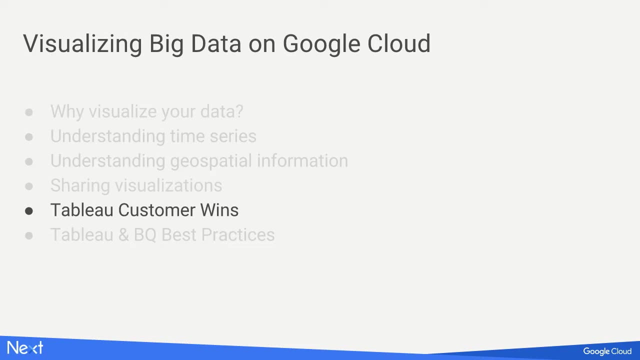 you want to look up the code I used to build these demos, But if you're not a coder, there's another option, and that's Tableau. Tableau is a powerful visualization and analysis tool, No coding skills required. And to show you more about that, 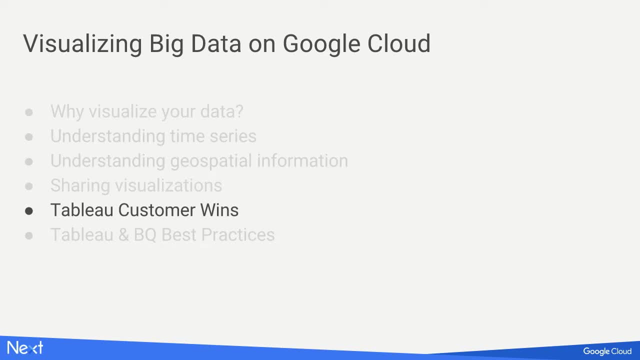 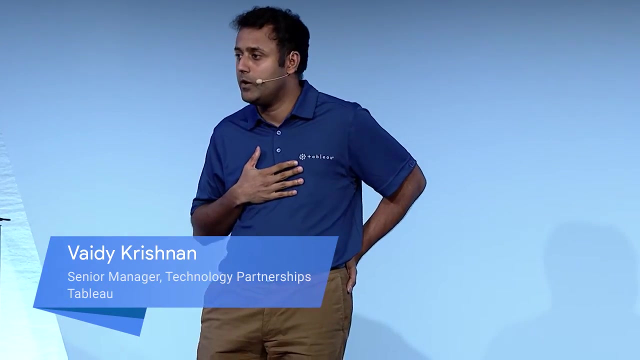 Let me introduce Vaidhi Krishnan, who's going to come to stage and show you how GCP customers are using Tableau to gain insights about their big data. Thank you, Of course. So my name is Vaidhi. I lead partnerships for Tableau, so my job at Tableau is to work with Google and all 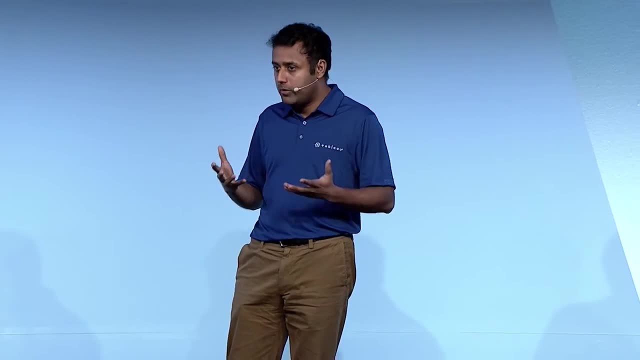 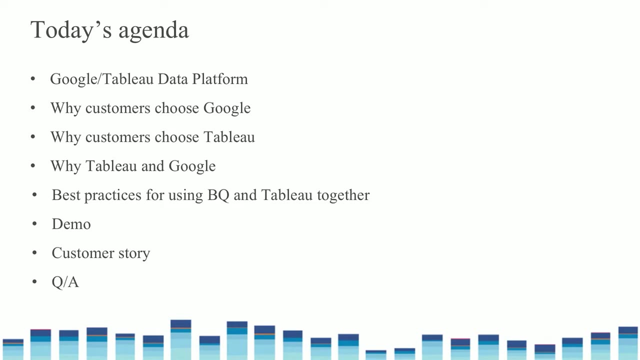 the other technology partners we collaborate with and that help our customers be more successful with Tableau, And today I'm going to talk to you about, First of all, how Tableau integrates with the Google platform, why customers choose Google, why customers use Tableau and why the joint value that we provide is a win for. 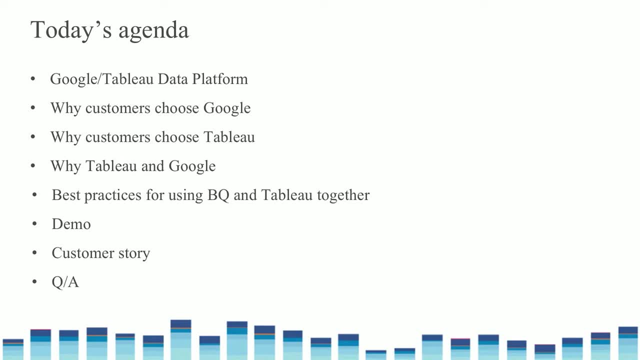 both of us and our customers. Then we're going to get into some best practices for using BigQuery and Tableau together. But before that I just want to you know, do a quick show of hands. How many are familiar with what Tableau is? 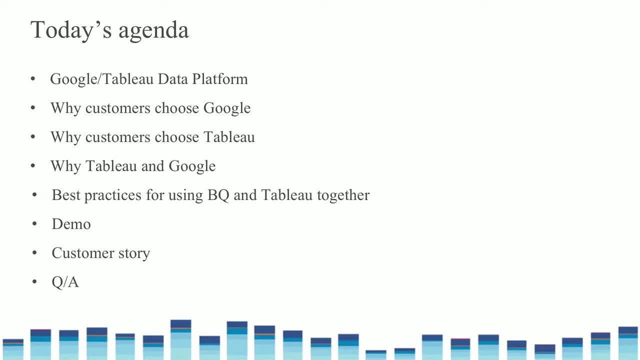 Or are already using Tableau, So that's great right. So it seems like everyone has had a chance to you know, experience Tableau or are already using it, But I'm sure many of you have sometimes struggled with performance and haven't quite understood. 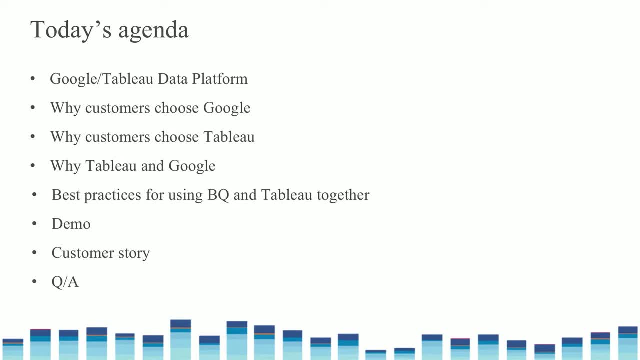 how to work with that And we're going to talk about some best practices. And before I will end, I'll just get into a quick demo where we'll connect to a billion rows worth of data And I'll talk about some big customer wins we've had, including, you know, several that. 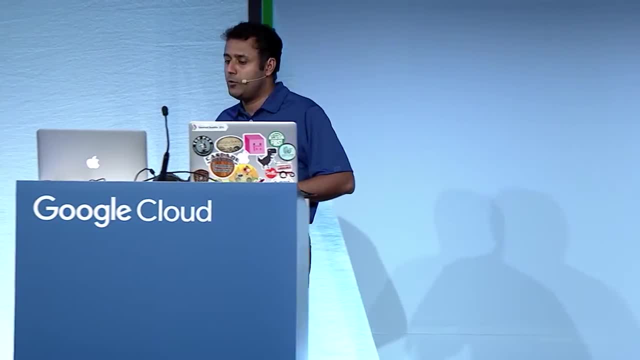 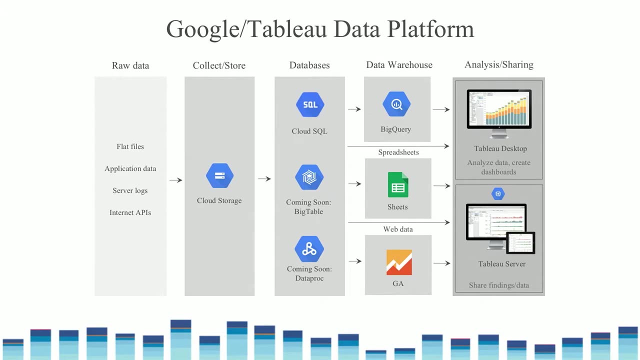 were featured on the keynote stage yesterday. So here's what the Google Tableau data platform looks like. So Tableau is just a top layer of a very deep stack that most customers use to organize and analyze information inside their enterprises. So Tableau is just a top layer of a very deep stack that most customers use to organize and analyze information inside their enterprises. 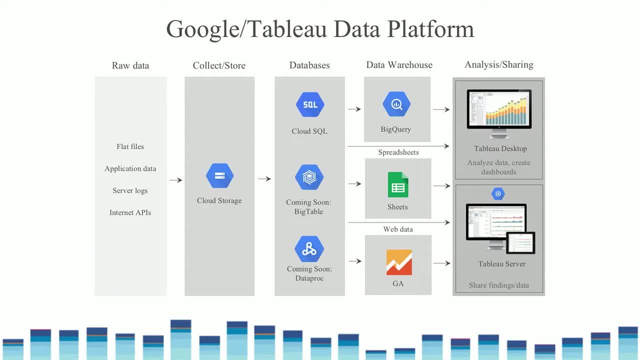 So Tableau is just a top layer of a very deep stack that most customers use to organize and analyze information inside their enterprises. So the way this works: in most cases you have some raw data. This could be, you know, coming from sensors. 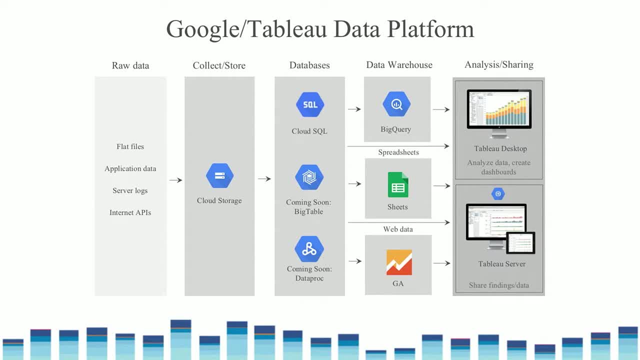 This could be sales, This could be marketing data. It goes into Google Cloud Storage, Then it flows into one of many different databases, all of which Tableau offers direct native connectivity to. So we're talking Cloud SQL. you know all of the marketing website data. 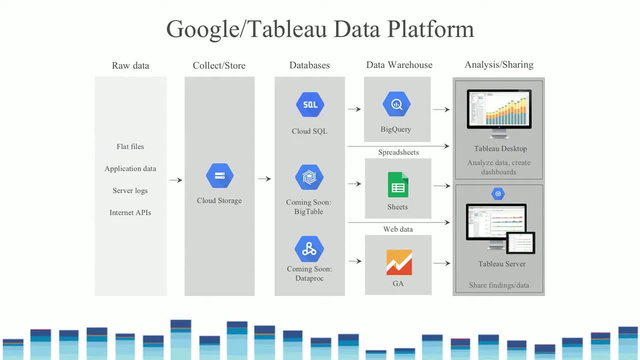 goes into Google Analytics, Google Sheets, Google BigQuery, So we'll talk about all of the different mechanisms that Tableau's got. So the way this works. in most cases, you have some raw data. You'll soon offer direct connectivity to Google Bigtable and to Cloud Dataproc, which 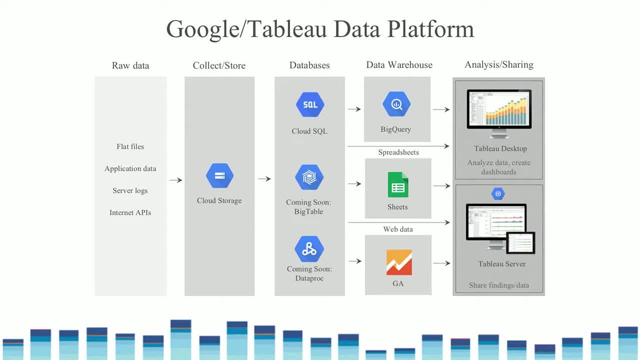 is Google's Hadoop as a service platform. Now many of you might ask: well, what is native connectivity? So native connectivity is essentially Tableau and Google working together to make sure our connection is tuned for performance and makes full use of the Tableau feature set. 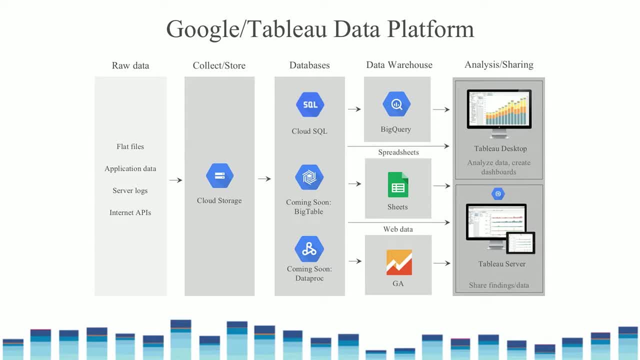 When we just connect via ODBC, it's not always optimized. So we have put, or both our engineers have been hard at work to make sure this integration is performant and works great for our customers. So we're talking about Google BigQuery today. 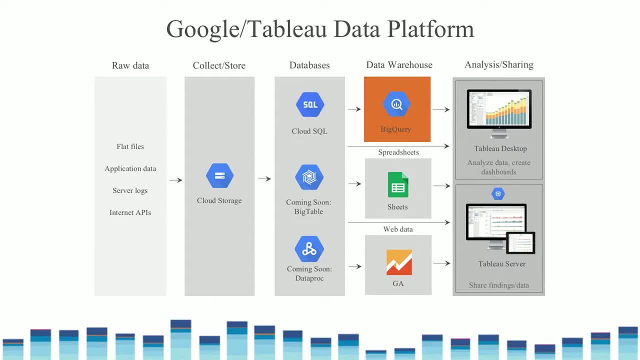 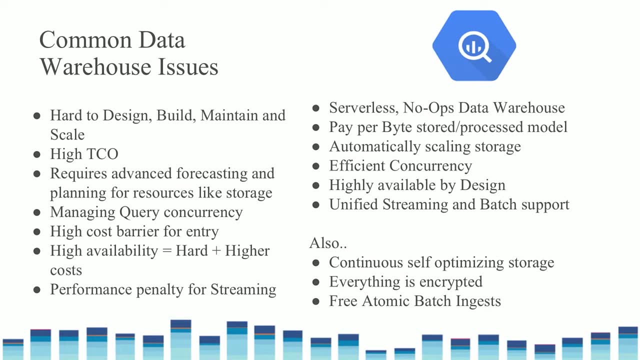 I want to spend a couple of moments just to emphasize why our customers like Google BigQuery- And I'm not going to dwell on this because I'm sure many of you have attended several other sessions that cover this- But what I like the most about the slide. 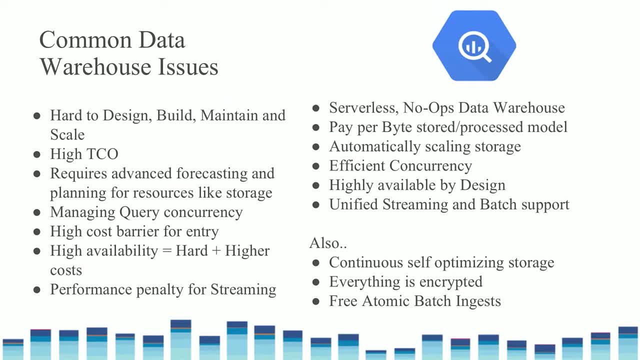 is that GBQ is doing away with all the traditional issues you face with data warehouses. on the left-hand side, You don't have to design, build and manage servers, You don't have to forecast capacity, And when you do that, there's typically a lot of total. 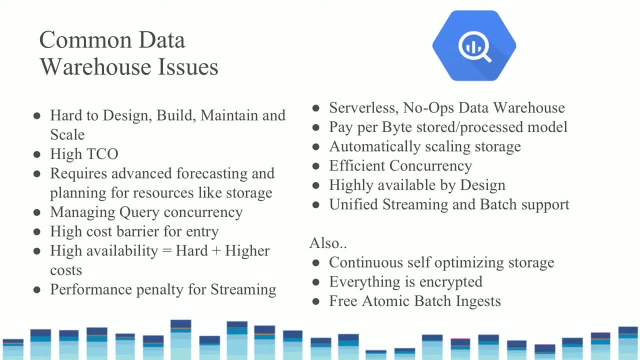 you know data. There's a lot of cost associated with it, which creates a barrier to entry. With Google BigQuery you have a serverless architecture, So it's completely abstracted out from the customer. You can automatically scale storage up and down. 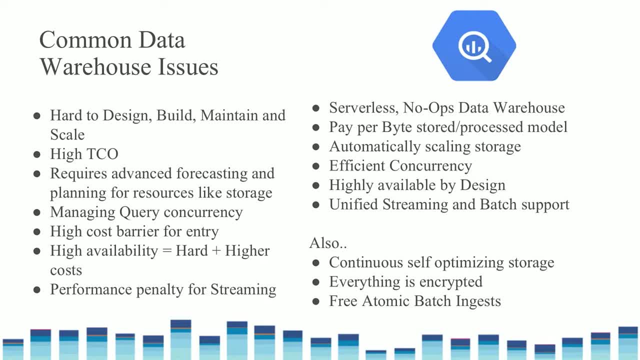 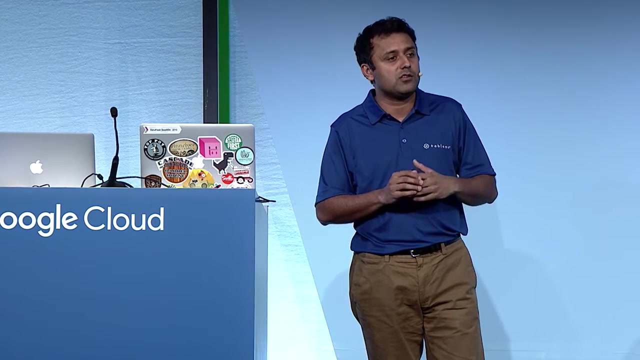 based as your needs and your usage grow, And you know in totality what this means is: the customer gets agility right, Like they don't have to necessarily invest upfront and deal with the risk of just letting their, or they don't have to deal with a lot of risks right. 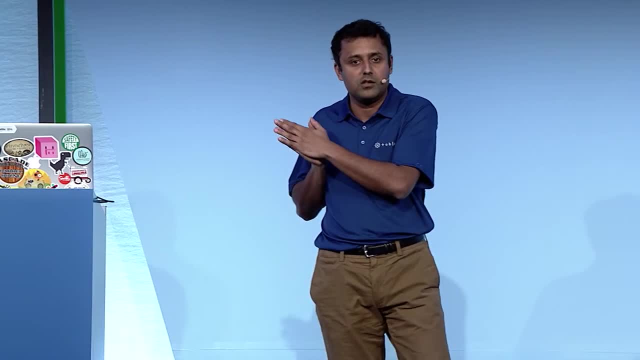 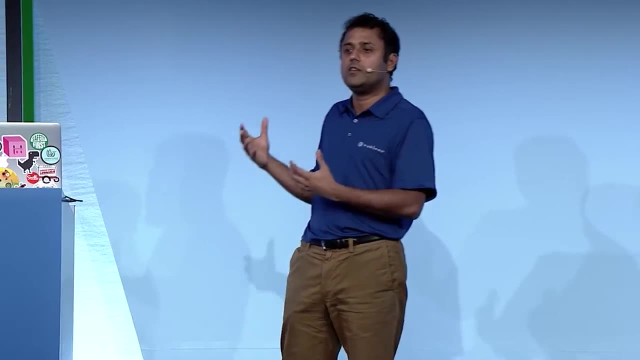 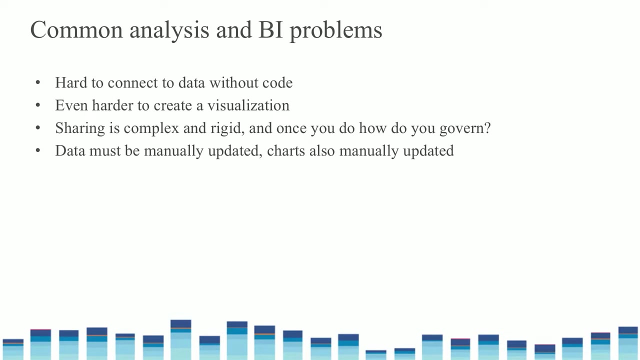 So, as with any cloud platform you have out there, Google BigQuery makes sure that they don't have to invest a ton in CapEx And most is OpEx and Scalable and Azure. So let's talk about some of the common problems you face with analyzing data. 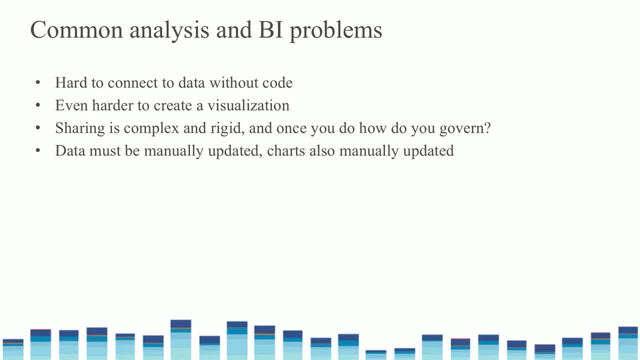 Well, first is, as with many legacy BI products and, in fact, a surprising number of new vendors, especially in the data discovery space, they make you write code to connect to data right, Which is great for a DBA or someone who's a developer. 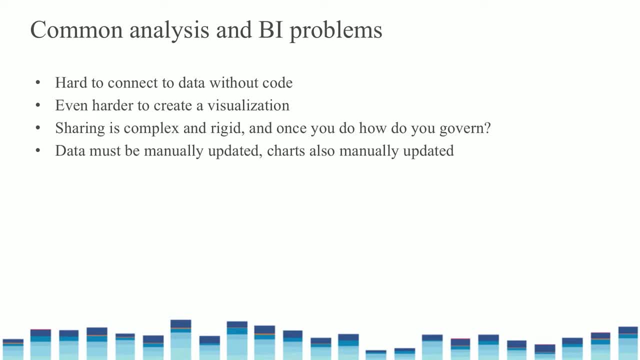 But if you're a business user or someone who is close to the actions that come out of his work and who knows the data, you don't have to spend time doing that Now. once you're able to connect the data, it's typically very hard to create a viz right. 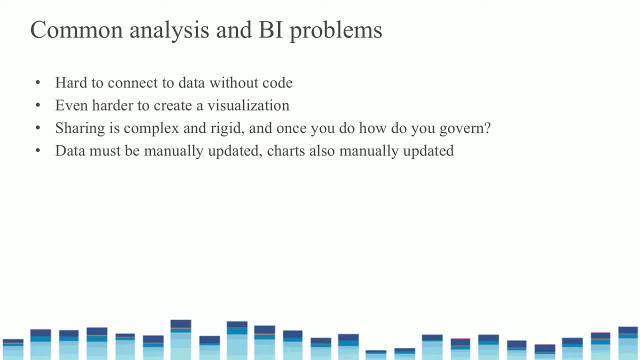 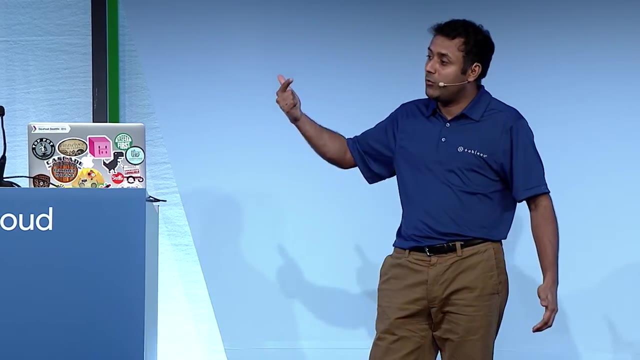 You need to know what question you're going to ask before you analyze data, But that's not how data exploration works. 90% of the time, I just have a billion rows and I don't even know what question to ask. I need to just explore a way and let that data guide. 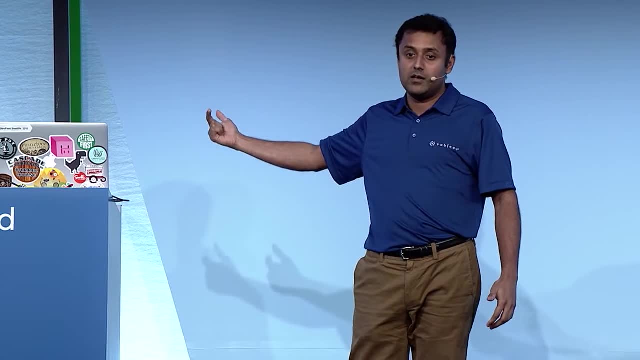 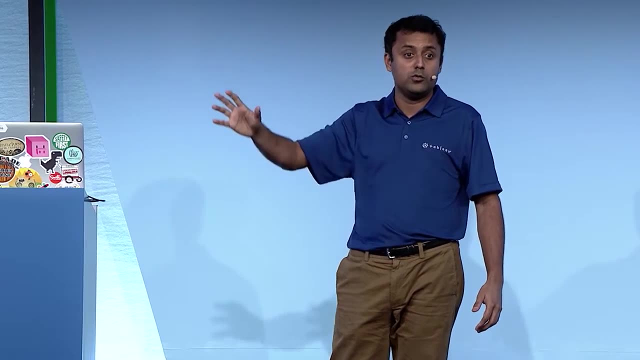 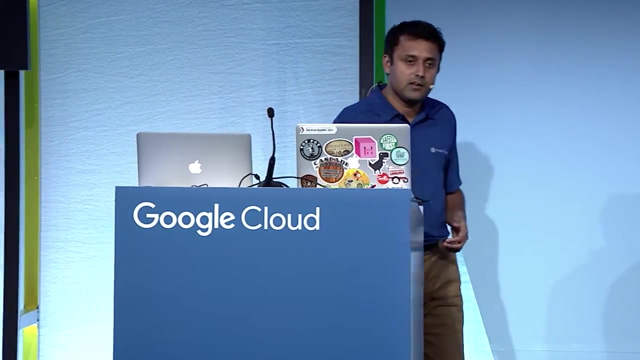 what that question should be. So imagine a platform that's asking you to click on a bunch of wizards or choose a chart type even before you've asked that question. We wanted to disrupt that experience, And I'll talk about how Tableau solves that. 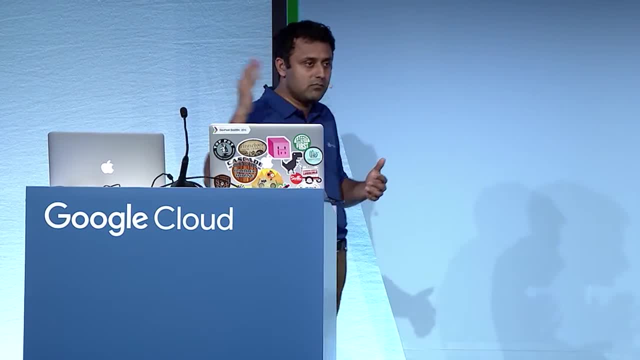 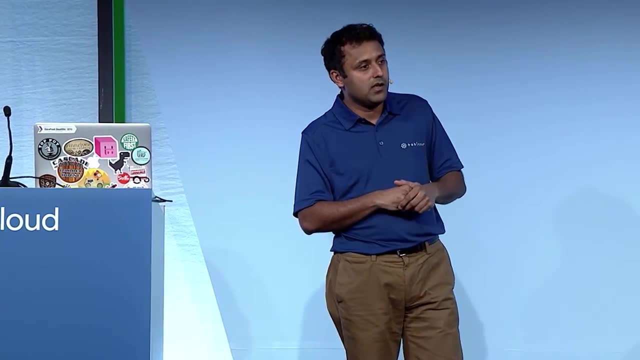 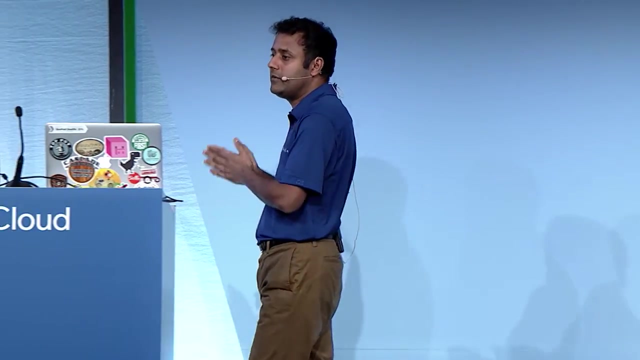 And finally, once you've created something you have to share- And Tim alluded to this a little earlier- Share that work with the rest of your organization. You know this could be internally with stakeholders or clients, to make sure that that analysis is acted on right. 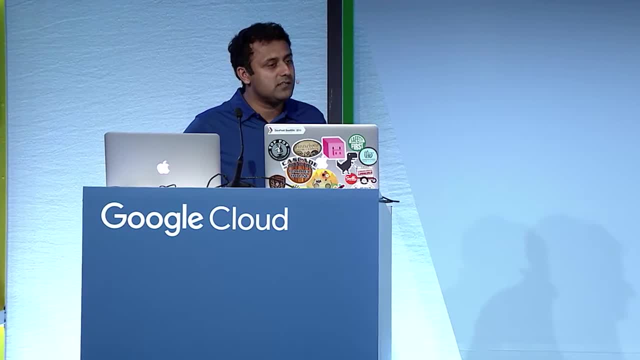 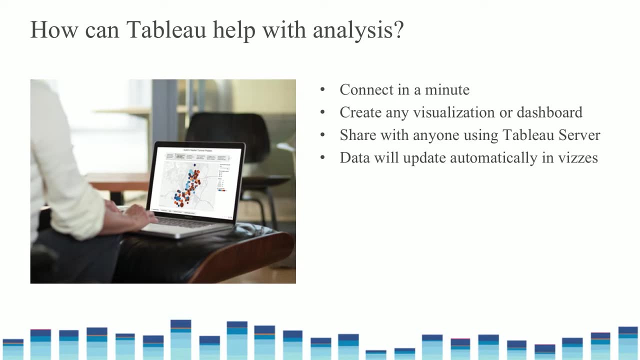 And again, that has typically not been easy in traditional BI platforms. So how can Tableau help? Well, first of all, you can connect to all the Google data sources I talked about, and a whole slew of other data sources, in a minute. 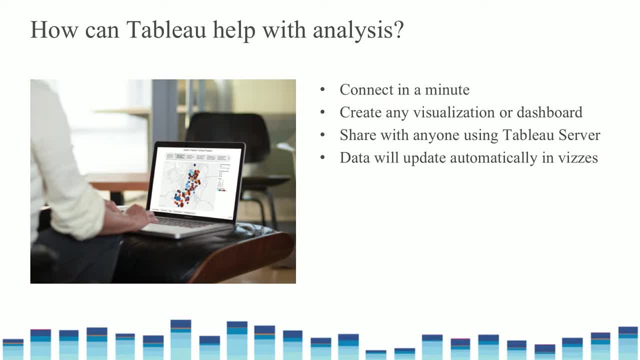 Right, And I firmly believe that, across most organizations, not all your data rests in one place, right? So you may have a ton of data in GBQ, but you have data in Salesforce, You have data in Marketo. You still have some of those old spreadsheets. 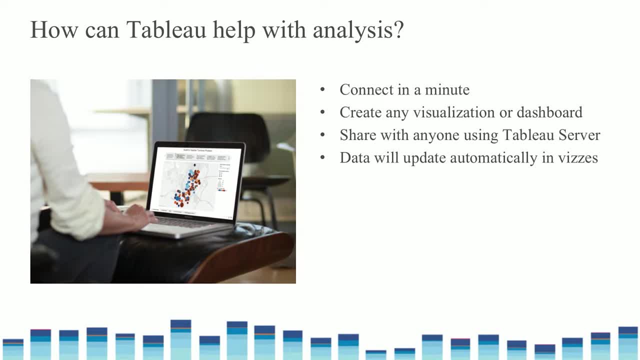 that some of your teams may be continuing to update on an ongoing basis that you want to bring into your analysis. right, We allow you to bring all those data sources together And we are not just a visualization, We're a tool. So I know when we started out back in 2003,. 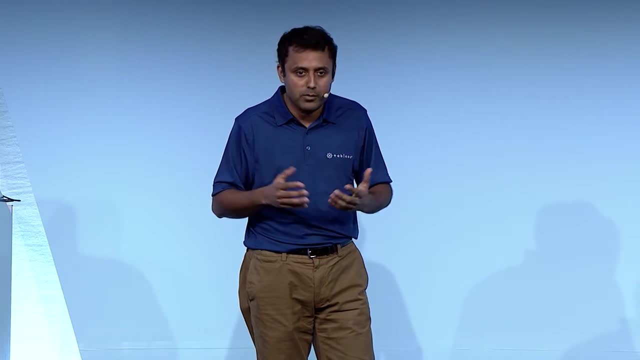 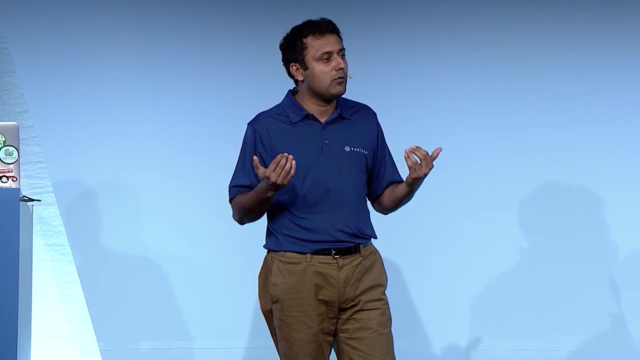 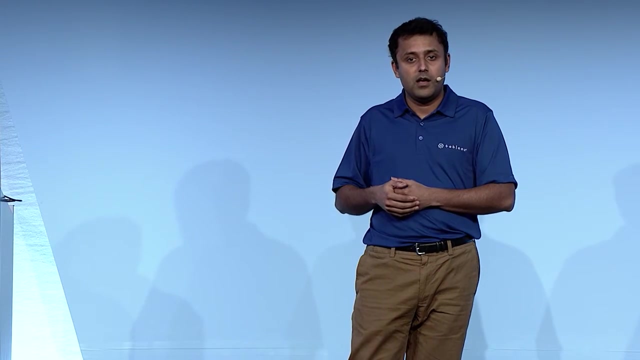 the first couple of years, the market saw us as a shiny new toy, But over the years we've expanded our capabilities. We're now proud to be an enterprise-ready mission critical platform that allows people not just to analyze and explore data, but to share, govern and 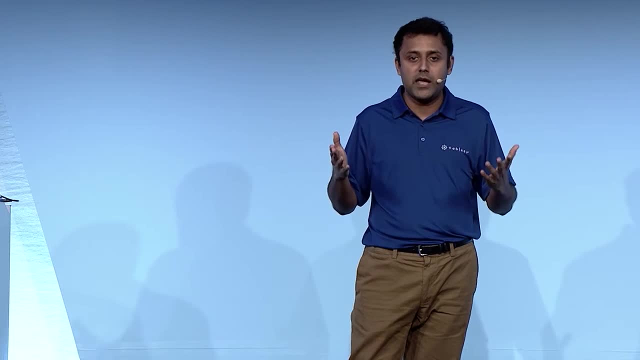 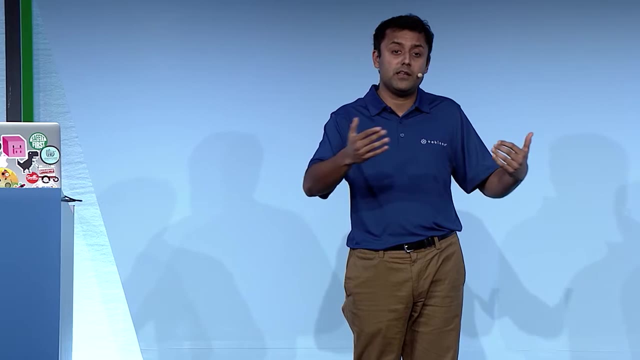 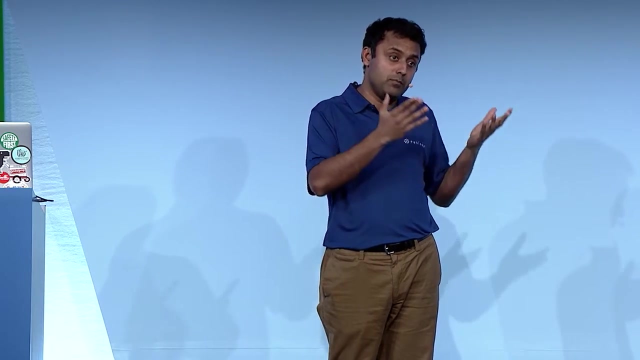 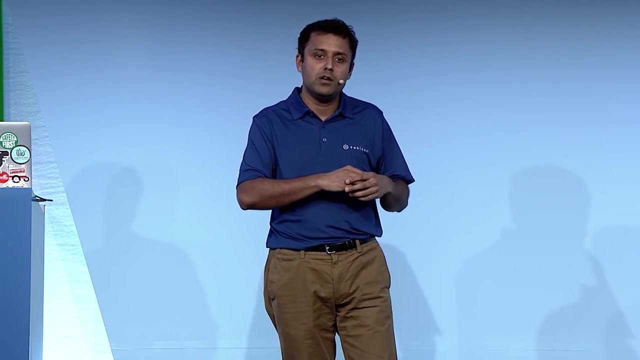 collaborate and distribute it in a way that makes people feel empowered. So, and IT can also participate now in driving the analytics direction of organizations. So your business users are governed without feeling that they're being governed, And IT is now able to focus all its time. 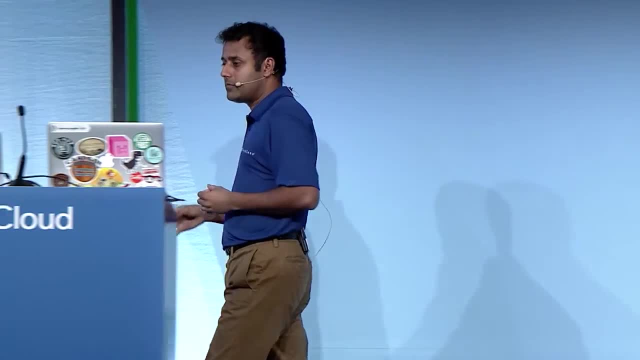 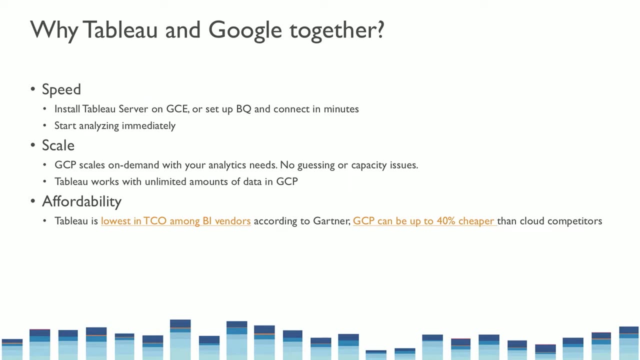 on high-level security and data management tasks. So how do Tableau and Google work together? Again, it comes down to three things: speed and agility. We deploy on the Google Cloud Engine. You can connect in minutes, start analyzing data right away. 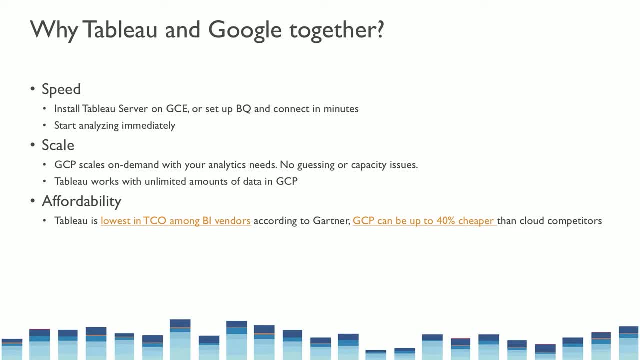 GCP offers scale and agility. There's no guessing capacity issues. You don't have to forecast in advance. Scale up and down as you need, And Tableau works with all kinds of data and unlimited amounts, And I'll illustrate that in a demonstration in a little bit. 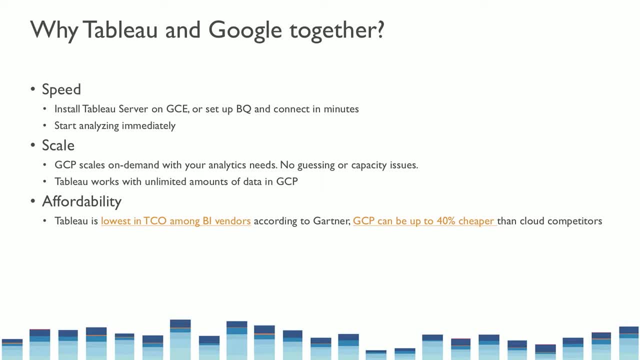 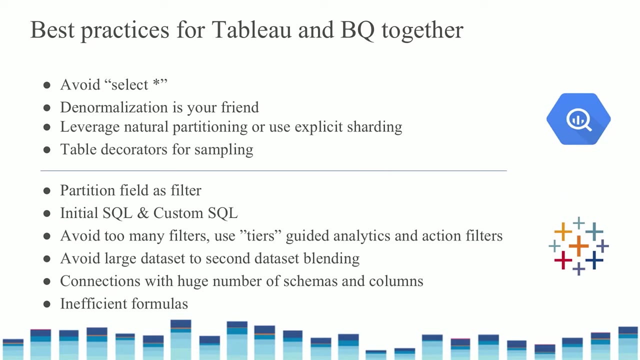 And of course, there's TCP. TCO, which both of us are really great at. Ours has been ranked the lowest among all the major BI vendors, And GCP can be up to 40% cheaper than cloud competitors. So what are some best practices for Tableau and BigQuery? 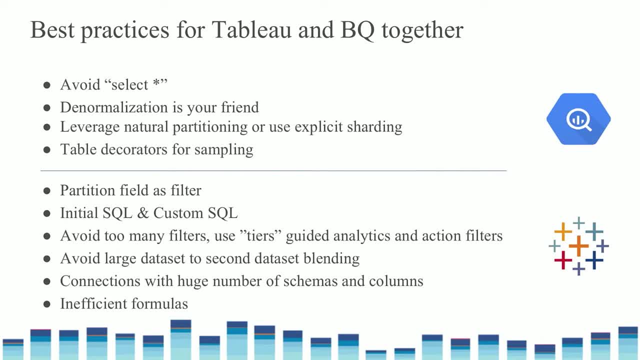 together Again. I'm not going to dwell on all of these, but there's a few ones that I would like to just double-click on. The first and so the top half is all the best practices, but Google will teach you, too, what. 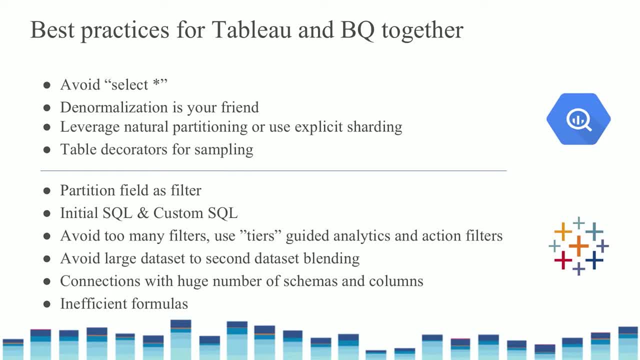 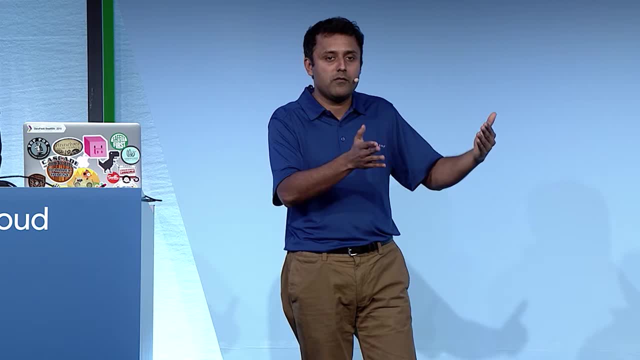 are some of the best practices that have to deal with Google BigQuery. So, first of all, when a visualization is not performing 50% of the time, or I would say 70% to 75% of the time, you haven't tuned your data source well. 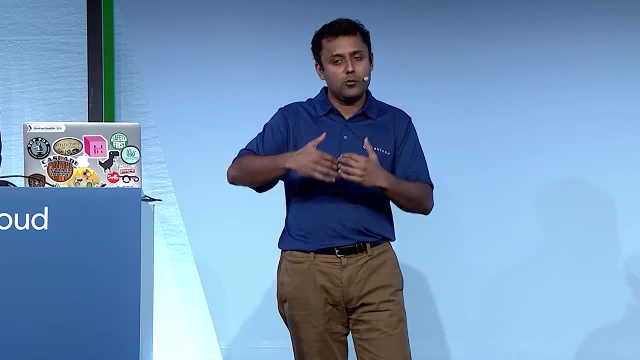 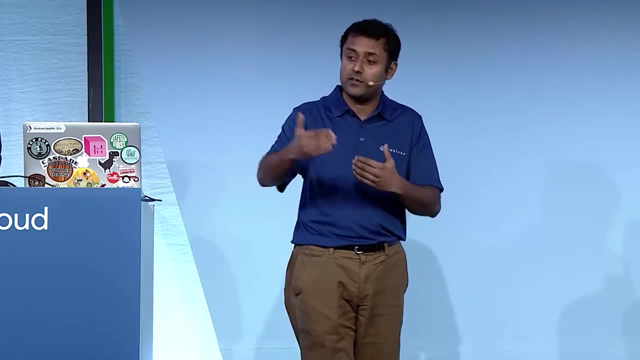 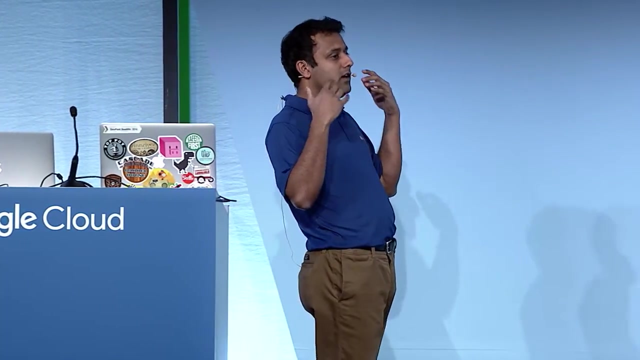 It's the data source that performs against the data source. I always like to tell my customers if your SQL against the data source is taking 50 seconds, Tableau cannot make that 40 seconds. So what do you do? Avoid select star. Why is that? Because Google BigQuery is a columnar. 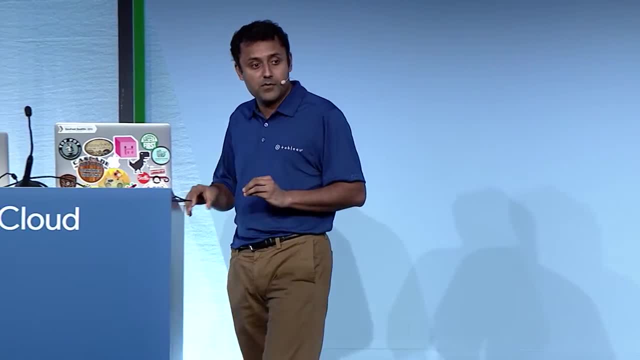 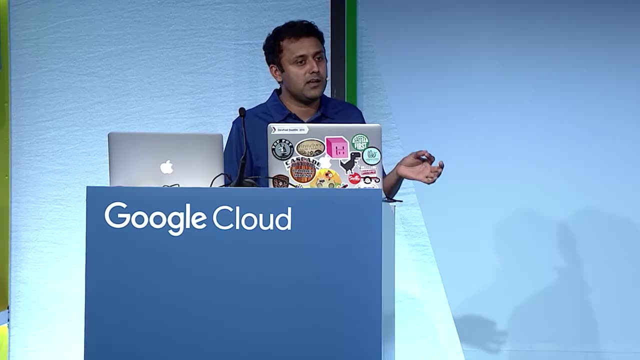 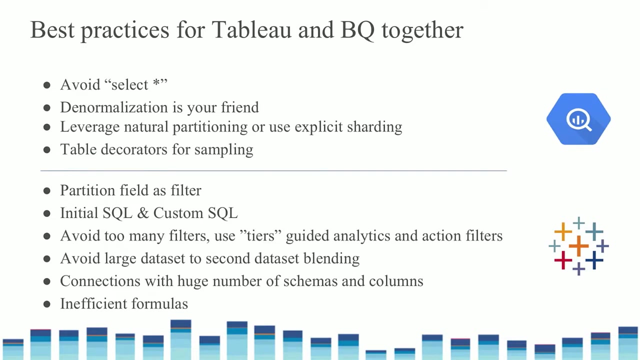 store. so what that means is every column is in a different physical block. So if you choose your columns and not do select stars, queries are going to be more performant. Denormalization is your best friend, So Google BigQuery is great at joins, but if you're able to pre-join, 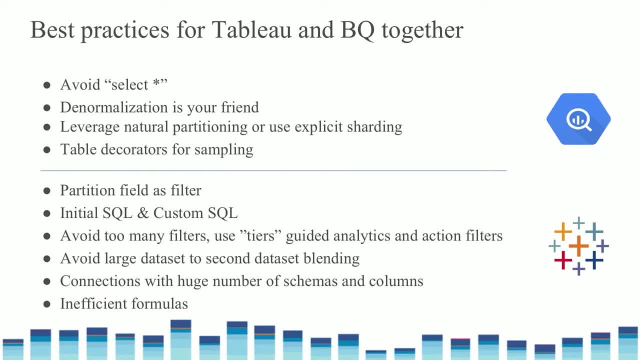 and flatten out your structures. and you know, essentially, you know- trade your storage for compute resources. well, obviously you're going to be paying more for storage but paying a lot less for compute, and I think that's a very effective tradeoff. Your queries are: 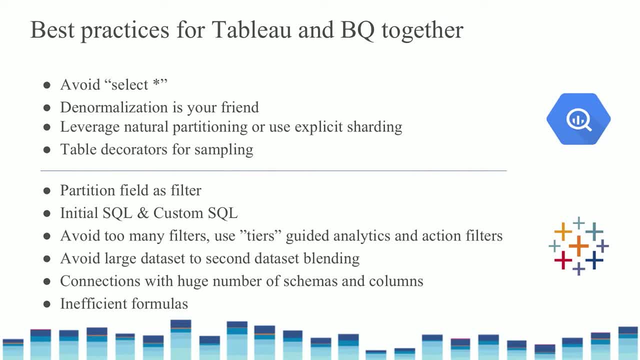 going to come back faster. So always denormalize your tables, and actually this works for Tableau as well. We like denormalized structures because it helps us fire that analytical query a lot better. Leverage natural partitioning or use explicit sharding. So again the point. 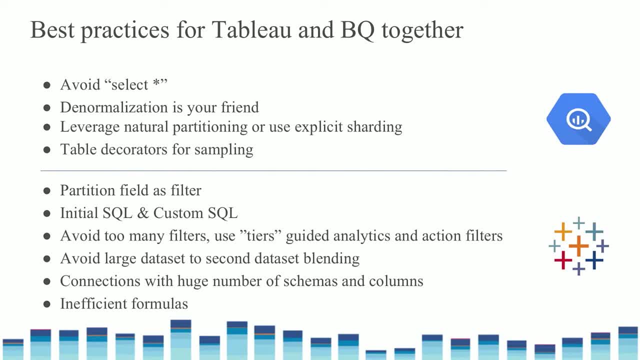 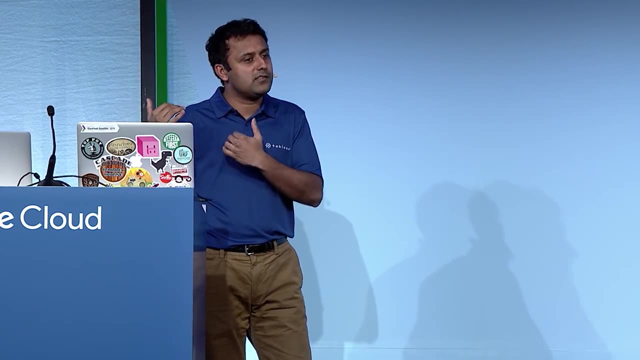 we're trying to make is avoid full table scans, So, and leverage natural partitioning, which is usually your record create date. So if you have a bunch of tables and you have one table for each date, you can use that or, you know, make sure you're using some sort. 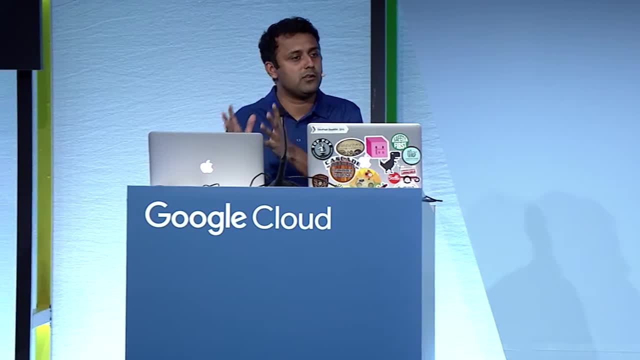 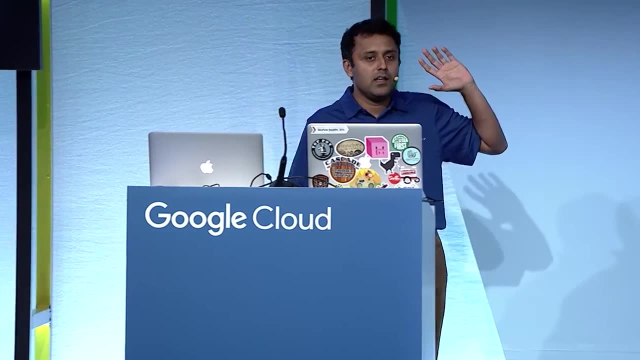 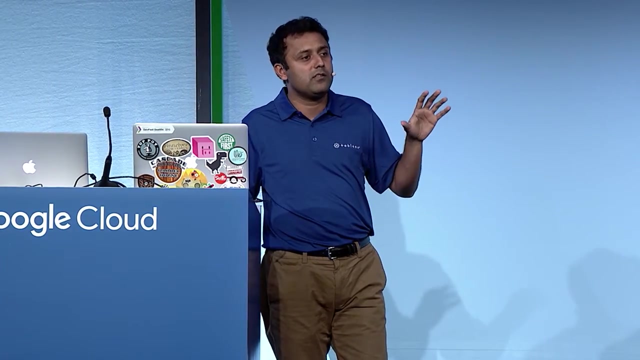 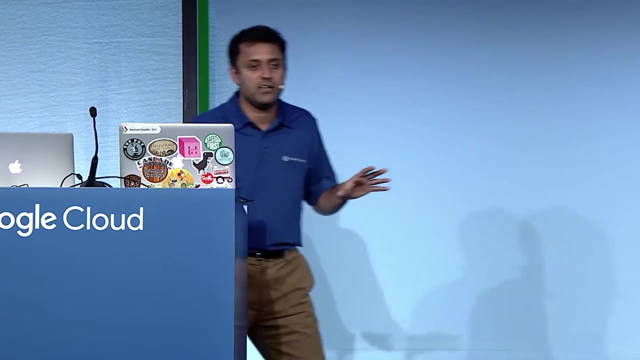 of filter to not scan everything and just scan what you need. On the Tableau side, you know again, I have seen billions of rows' worth of data. you know experience- or people experience 20x performance improvements over several billions of rows of data just because they had a solid indexing and partitioning strategy. Avoid. 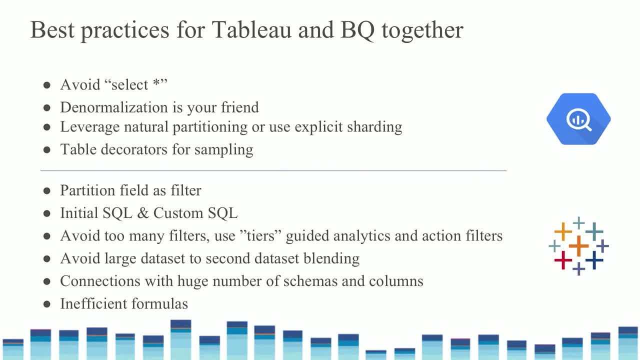 too many filters. Avoid large data set to second data set blending. You know, the thing about Tableau is just because it's easy, it allows people to do that And it's not just for people to do a lot of things. And just because you can do it doesn't mean you should. 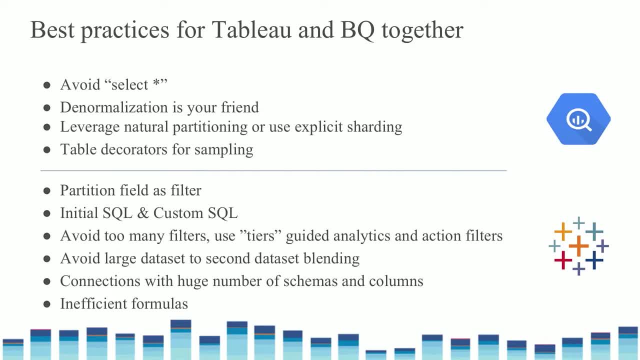 So avoid that And, you know, stay away from having large number of schemas and columns. You know it's always good to know in advance, or try to figure out, what are the columns you want to explore versus what's junk. And only you know connect to what you know for. 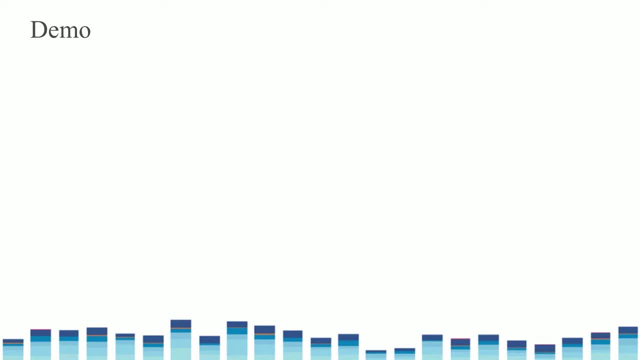 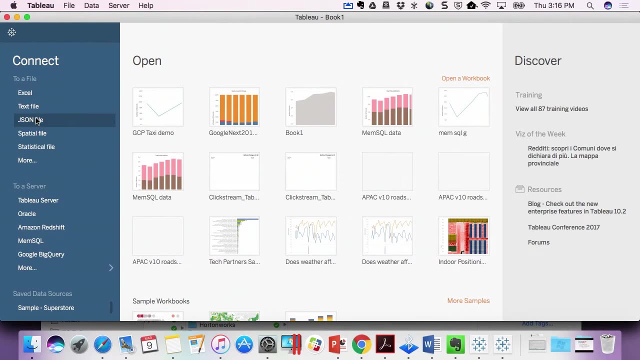 sure you're going to use. So, with that, let's get into Tableau. So let's get into a really quick demo Here. I am connected to Tableau desktop, So this is what an analyst would use to create visualizations, Right? So this is the analyst And I am going. 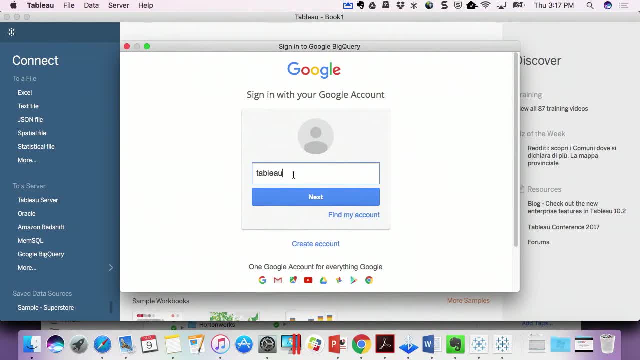 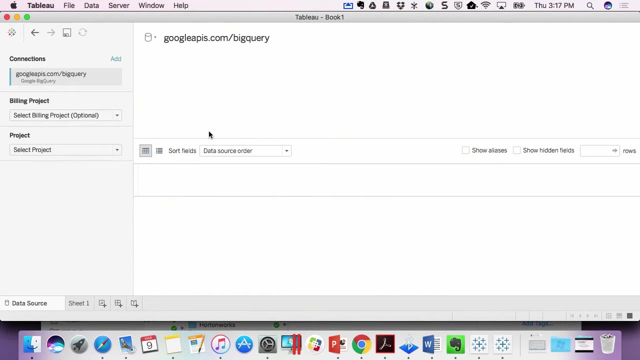 to go ahead and connect to Google BigQuery instance Five minutes- And I want to highlight some of the improvements we've made recently, you know, in support of some features that the Google BigQuery team have developed. The first thing is, since GBQ charges for storage and compute separately, you can now use the billing project feature. to point or to charge a certain project in a particular string. So that's a great feature. That's a great feature to be able to use if you want to be able to do that. So now you just have the discounts, you got some discounts And you can go ahead and connect with your team And then for us, instead of going to Google BigQuery. you can connect to Tableau by using a standard user keyholder index name. You can use the billing project feature to point or to charge a certain project in the file. 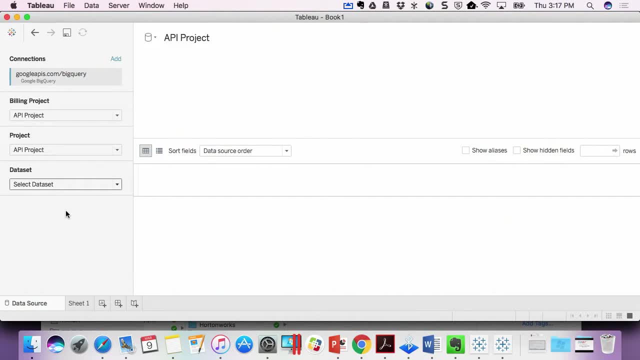 And this is actually only a general benefit of that. So there are your different features, So you can project. So imagine you have a bunch of stakeholders or clients. You can actually charge all the queries to that one project, which saves a lot of headache down the road. 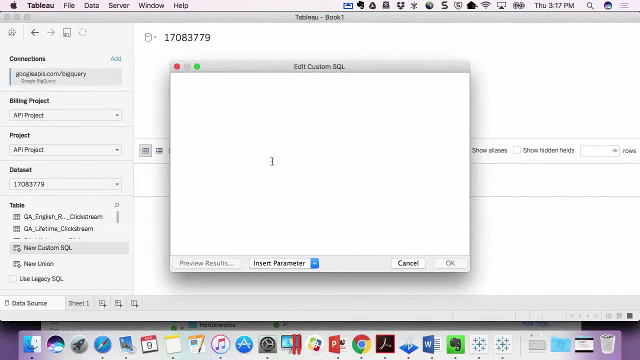 The second thing is we have now the ability to write custom SQL which can be validated right away. Why would you want to write custom SQL? A bunch of different reasons. Sometimes, for instance, you might want to use a native Google BigQuery function. 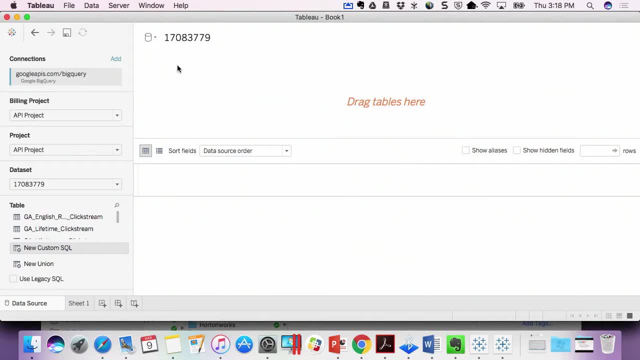 Let's say you want to use the wildcard function- How many of you are aware of that- where you can actually do select star from table dot star. So if you want to do something like that, you can leverage custom SQL. Also, we have added a little flag. 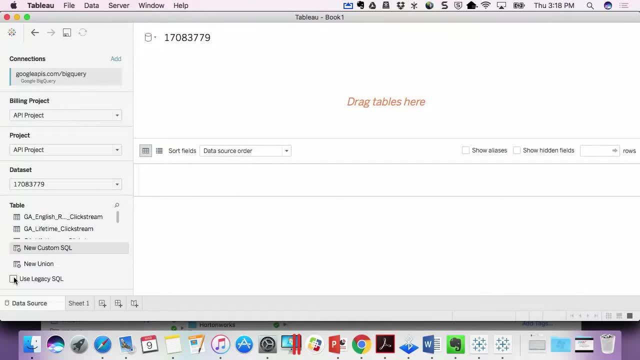 that lets you control whether you want to send a legacy SQL or standard SQL. So GBQ has now announced support for standard SQL, which is anti-SQL compliant. But there are several customers who have views that have all been written in legacy SQL. 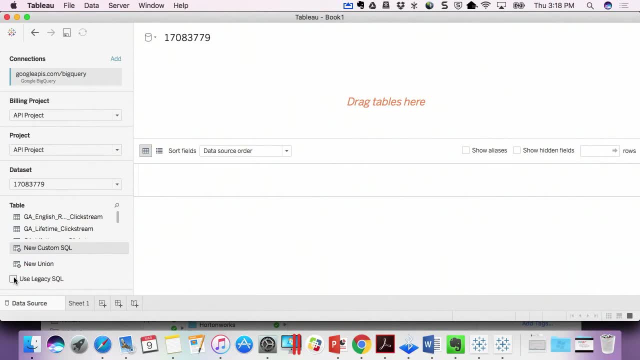 So when that's the case, you obviously want to send legacy SQL, and we give you that option. So let's go ahead and do some analysis. So here I am going to pull. I think it's about six or seven years worth of New York City taxi. 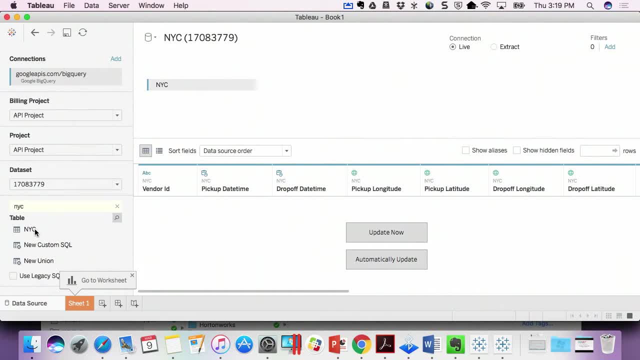 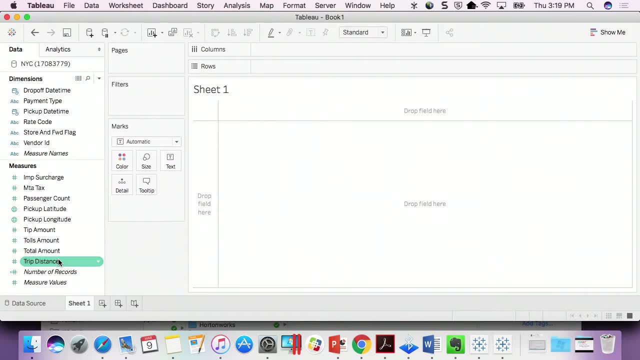 data All downloaded from the nycgov website and staged into Google BigQuery, And I'm going to start asking some questions. The first thing I want to know is, well, how many rows there are. And let's do that. I think it looks like there's about a little in excess. 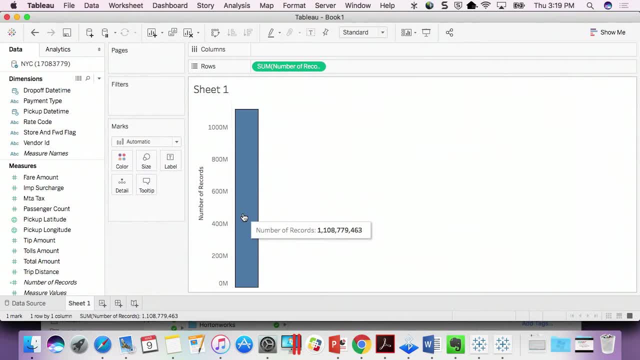 of a billion rows, And this is a perfect example of an analysis I'm going to do where I don't even know what to ask. Well, I'm just going to explore away. So first thing I want to know is: well, how have these number? 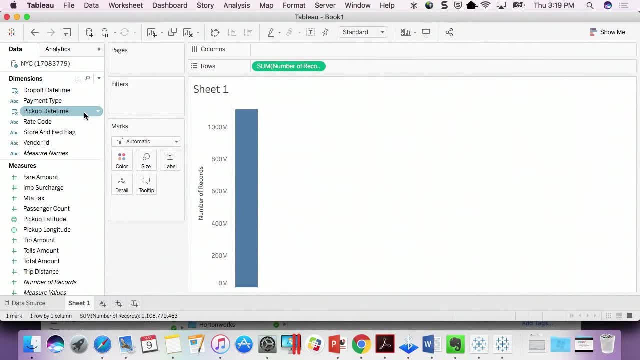 of records trended over time. So how about I look at this by the pickup date time And I'm going to look at this by year? Well, that's kind of nice. What if I want to look at it by quarter or month? 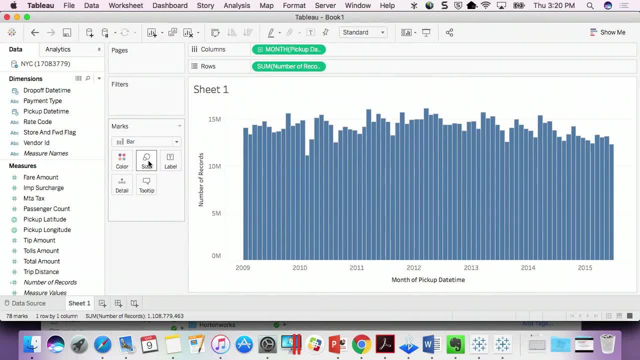 Maybe I want to express this a little differently as a bar. The other question I might want to ask is: well, how have the volumes of rides changed over time by payment type? So that's one dimension that I see in the data I have. 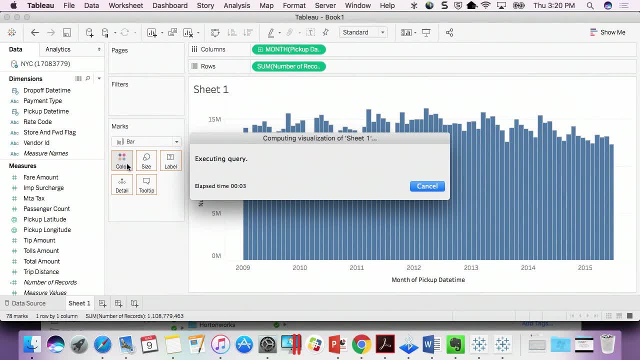 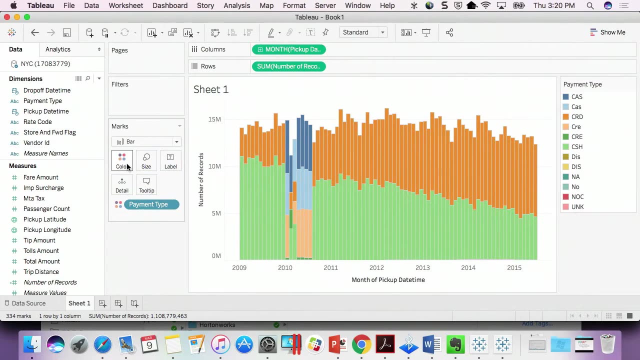 So I can bring that into color And it's going to fire that query again And hopefully it comes back in a bit. Now, while that happens, let me also tell you that Tableau is. it takes a hybrid approach towards data. 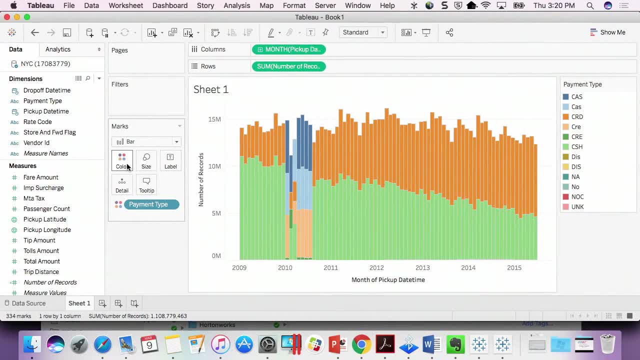 So we allow our customers to connect live. But customers are always encouraged to use our Tableau data extract if they only want a snapshot in time So they can always bring data into memory. And we have a lot of customers who may have trillions. 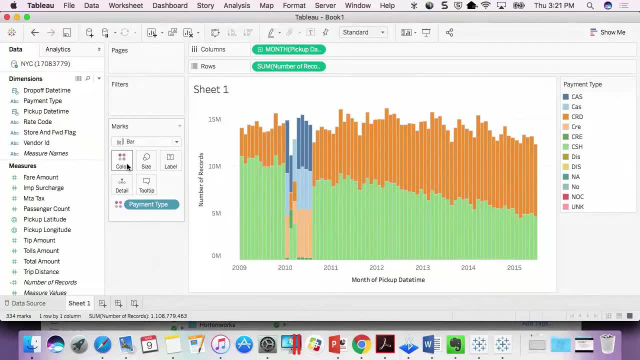 of records, But to prove a concept, they just need data for the last couple of years, And you can use a Tableau data extract to do that. So that's nice, And what this is doing is it's highlighting a problem that we see with a lot of data, which is dirty data. 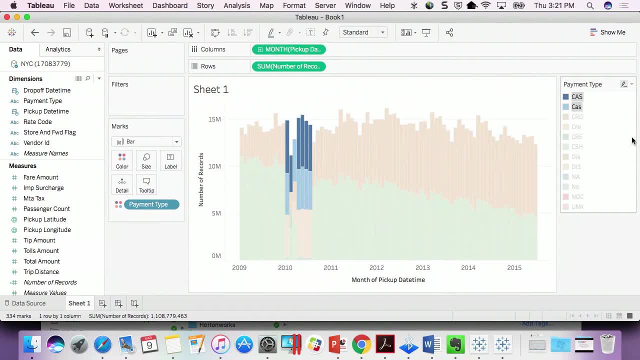 So here I have cash transactions being represented as multiple categories, So I might want to just go ahead and club them as one. So I'm going to do that right here, And when I do that, it doesn't change the source. All it's doing is it's changing the metadata. 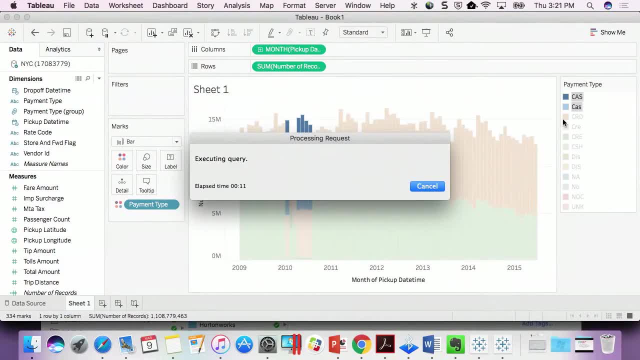 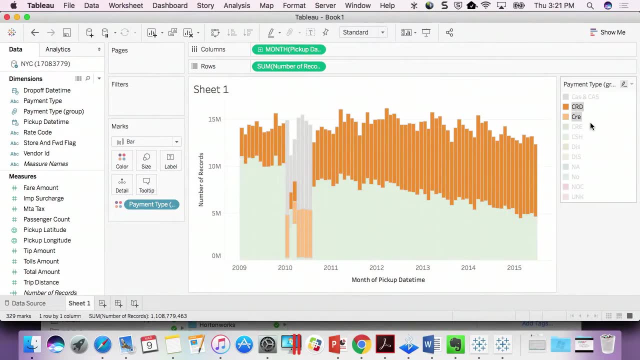 So now we will have a new payment group created. when that happens, I'm going to go ahead and club all the credit card transaction as one as well. So let's do that. So grouping that all into one, All right. So, and I'm going to keep the disputed transactions too. 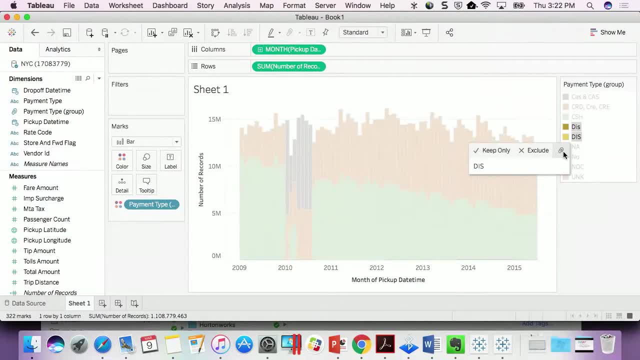 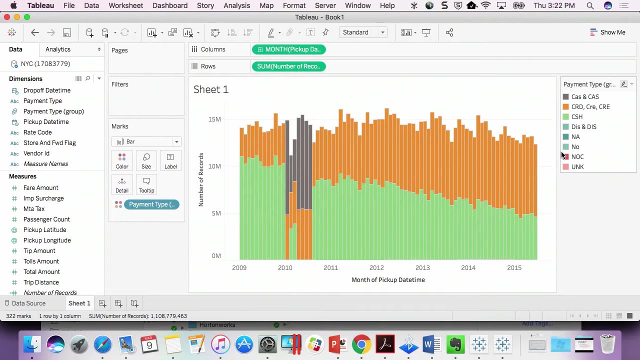 So, in fact, I think it might be useful to club that too, because that is something that I might want to analyze further. All right, So not surprisingly, if you look at the data from 2009 through 15,, the proportion of credit card transactions is: 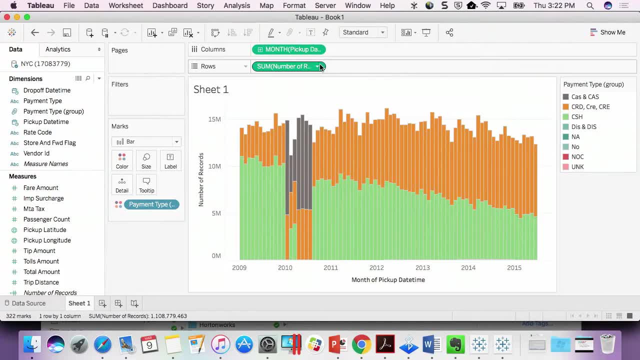 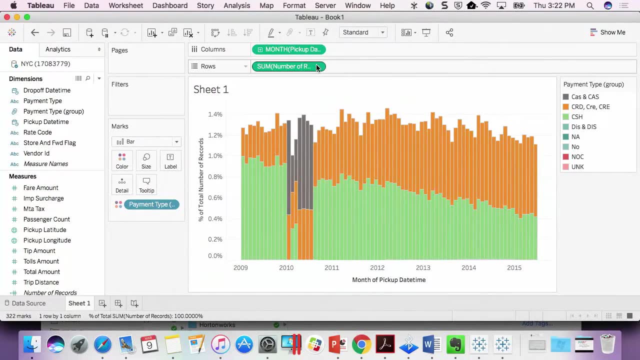 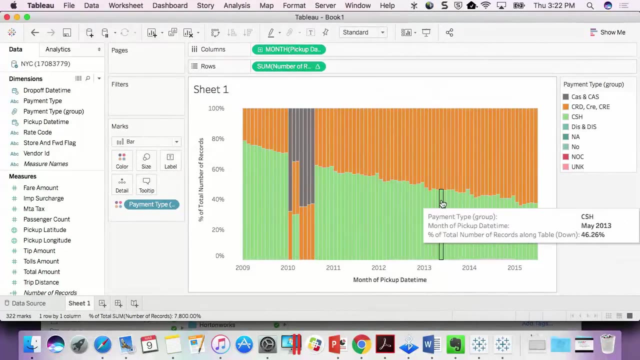 increasing And it's not all that surprising. But if you wanted to make the case a lot better, you can also add a little table calculation and express this result as a percentage of total. So that just makes it clearer a lot nicer. 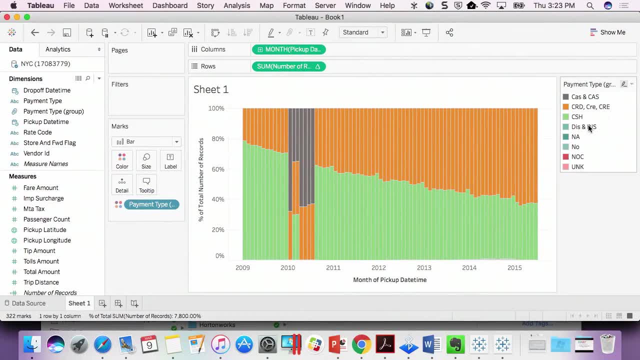 What I can also do now is ask a couple of different questions. So maybe I want to look at just the disputed transactions. Maybe I want to know When do all these disputed transactions happen And where do these happen, And does that tell me something about where these 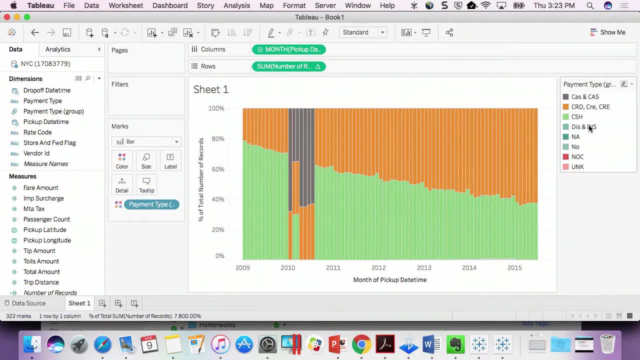 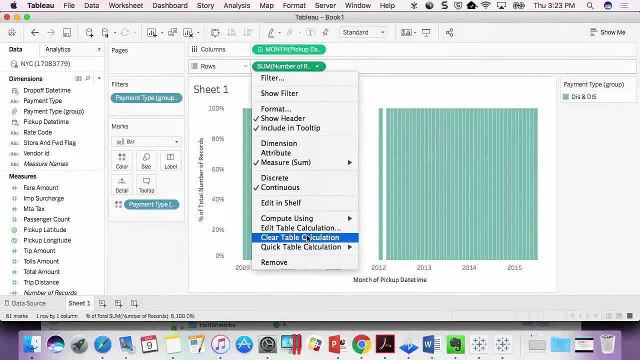 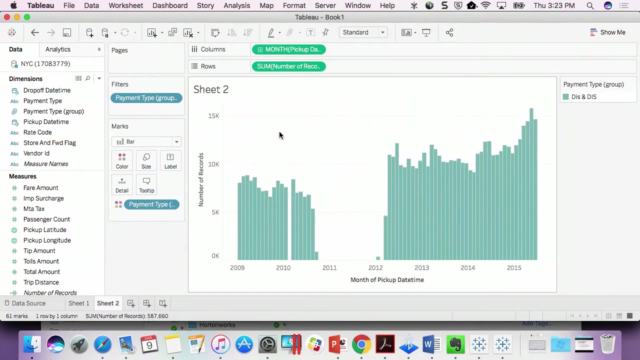 or where, as a cabbie, what are some areas that I might want to avoid? So I'm just going to go ahead and say, keep only, And I'm going to clear this table calculation, All right, And I'm going to go ahead and duplicate this sheet. 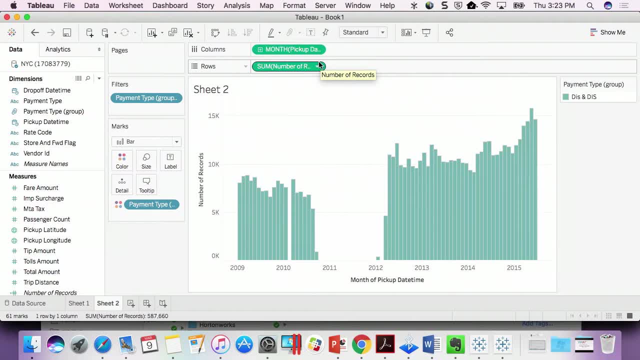 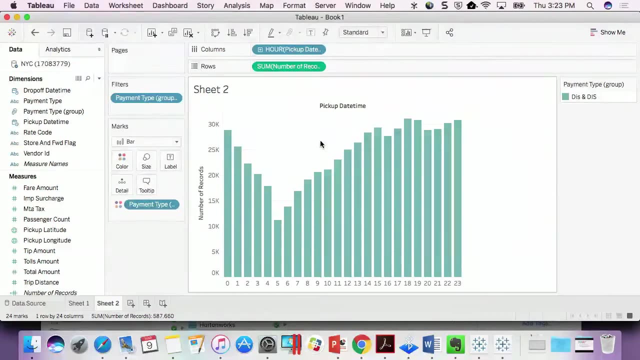 And now I'm going to try to express this data a little differently. Maybe I want to look at the same information by hour. Again, nothing surprising, Not a ton of rides happening in the wee hours of the morning, Right, But volumes grow as you get. 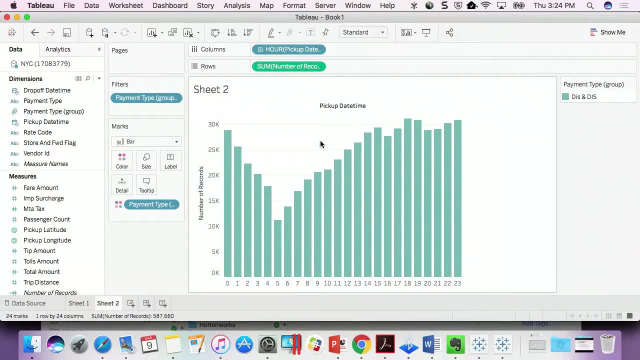 Later in the day. The next question is: well, can I hone in on certain neighborhoods or certain boroughs within New York where all these disputes happening in the wee hours of the morning? So for that I am going to represent this data geographically. 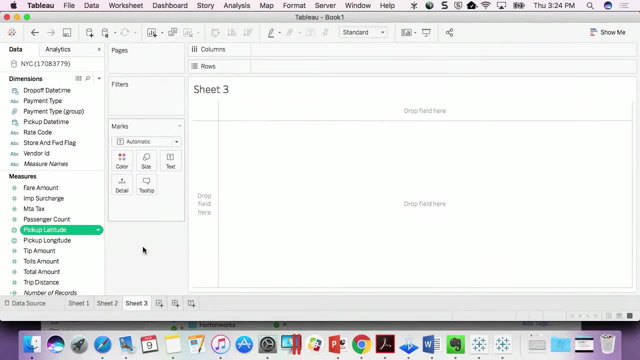 So let's look at my latitudes and longitude data. Oops, Oh, I got a mistake. There you are. That's what I wanted. That's my latitude, And let's bring in my longitudes here, And Tableau has automatically, by the way, geocoded this information. 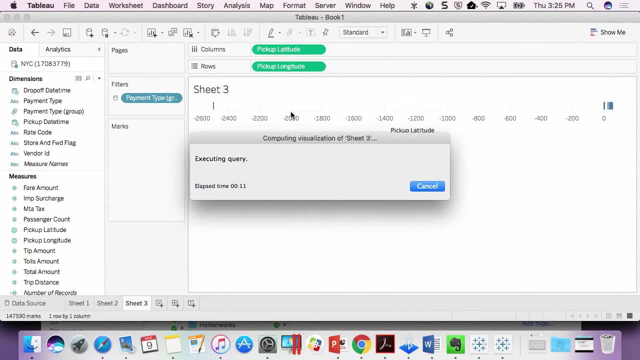 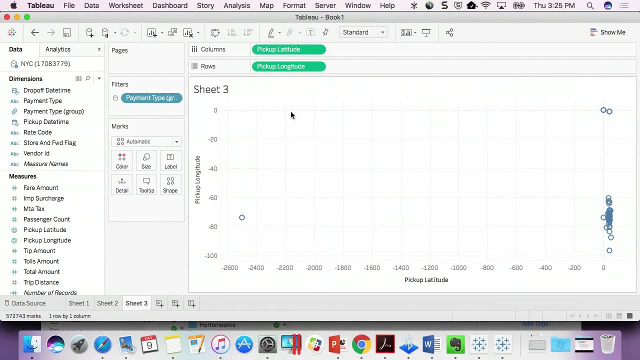 So it recognizes well-described addresses, It recognizes boroughs in New York, It recognizes zip codes. But if you don't have that, you can use a whole range of geocoding resources to bring latitudes and longitudes and actually have them inside Tableau. 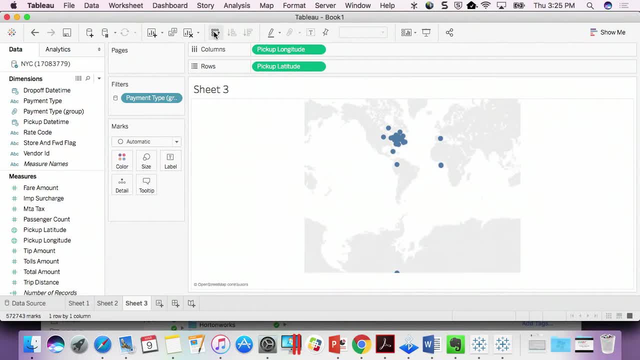 Now you see that there's some junk in here, which I mean some of those rights have been coded, as happening in Africa and Antarctica, and obviously I don't want that. So I'm just going to go ahead and hone in on just those rights that are coded correctly. 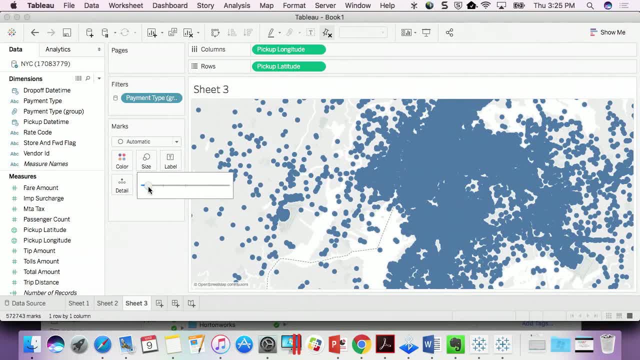 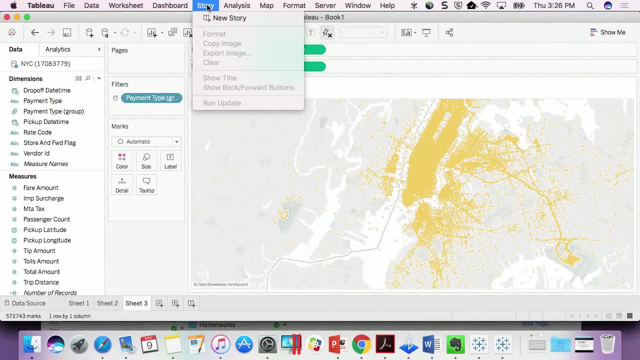 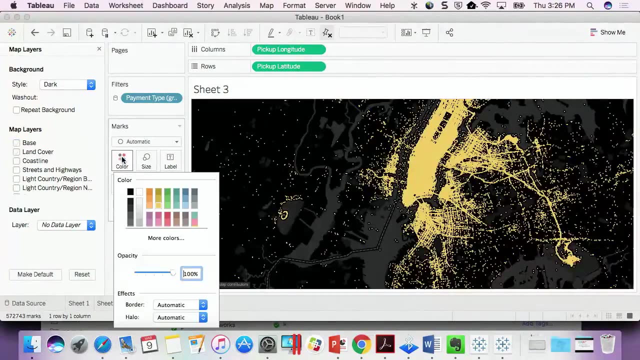 And that's a lot of rights. Why don't we focus in And just clean this up a little bit And I can change the map layer as well. That's nicer. And I can change the opacity, so it's nicer to look at. 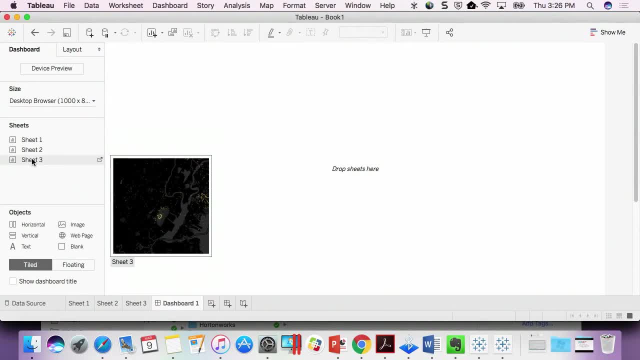 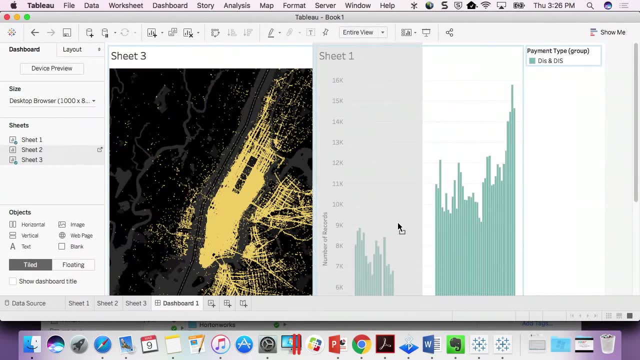 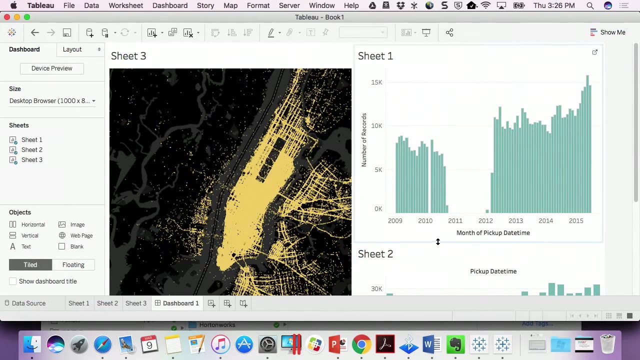 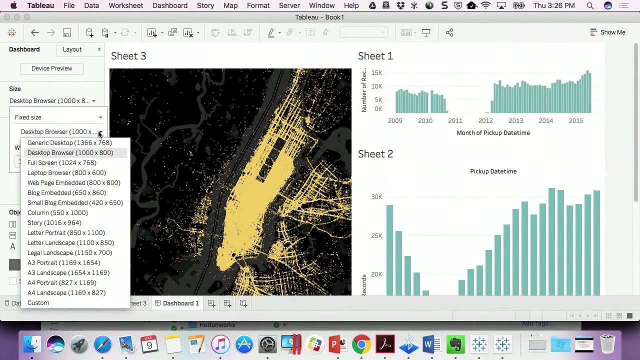 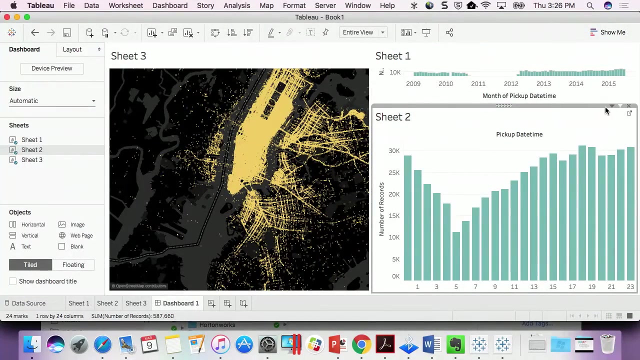 And now I can bring this all into a dashboard and actually connect these different views. Right, I don't need that. I can go ahead and make sure it's laid out right And I can enable action filters And with that I can use OneView to focus. 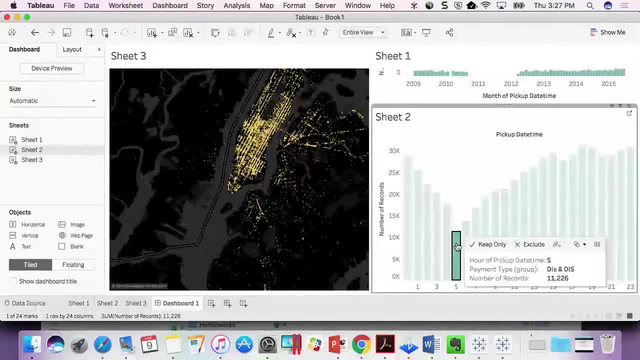 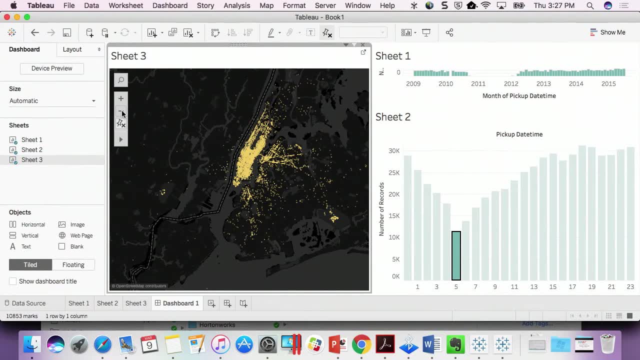 All right. So obviously we see here there's a lot of activity around LaGuardia, JFK, some busy thoroughfares around Brooklyn and Williamsburg, and Midtown is always crazy even in the wee hours of the morning. So again, just a very quick illustration of how all of this comes together. 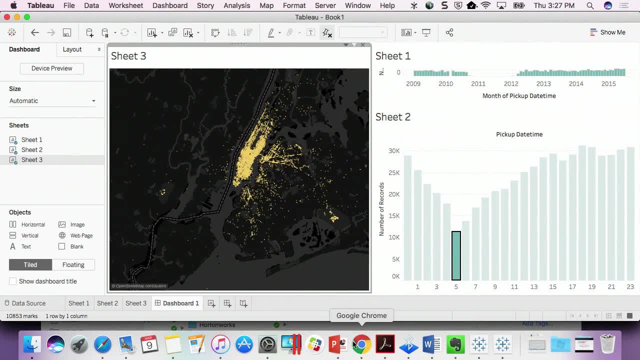 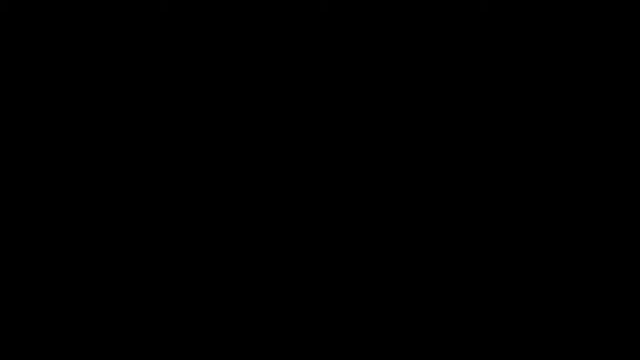 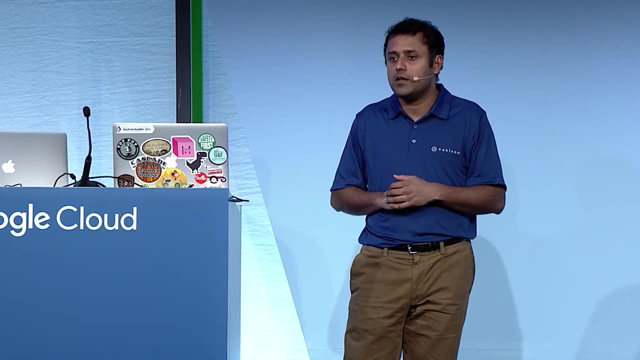 And again this was done off a billion rows. So how are customers leveraging Tableau and BigQuery together? So here's three different examples. We're a fairly horizontal platform. We have customers across all verticals using Tableau. We're in about 95% of the Fortune 500 companies. 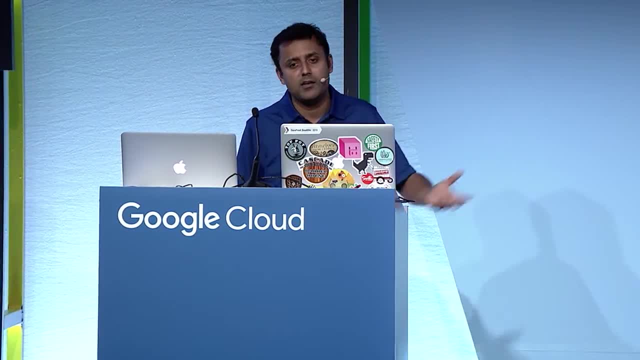 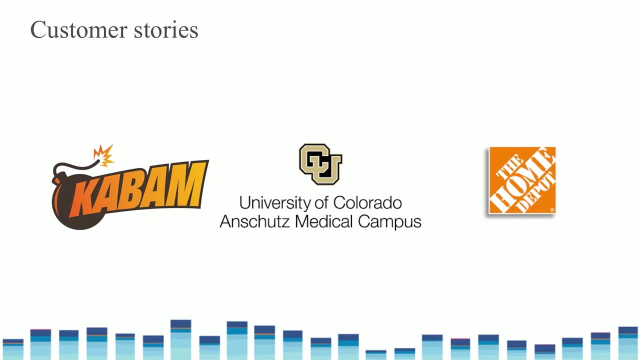 But the three I want to highlight are one which is Kabam, a very small gaming company. lots of data. They've had a relationship with Google, They've worked with Google, They've had a relationship with Google for years And they're asking questions around their gaming data. right. 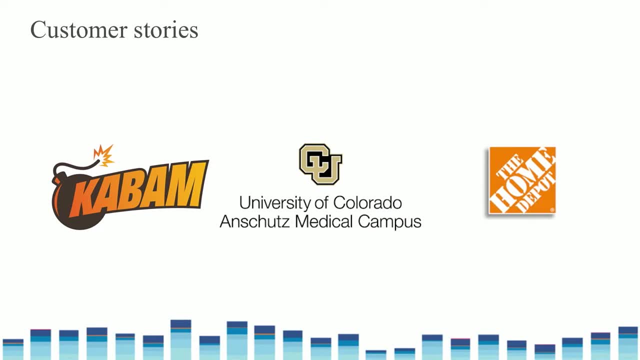 They want to know user behavior. Where do people get stuck? What are some? you know, how do I design the game so people spend more? These are the kinds of questions they're asking. You have University of Colorado at Denver, and they just came out with a press release. 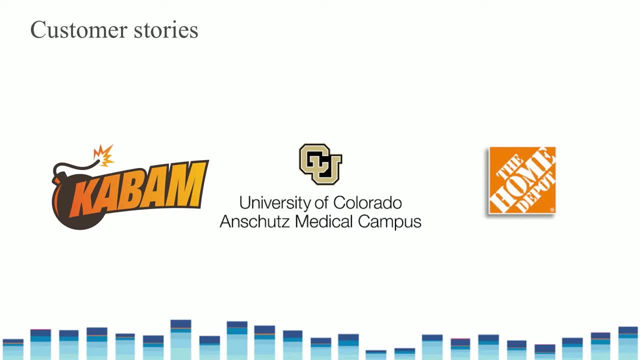 today They're bringing in their EHR data, combining with patient data and environment data to deliver personalized medicine. And of course, I'm not going to go into too much detail. I'm going to go into a little bit more detail. I'm going to talk about HomeD, but you guys heard from them on the keynote stage yesterday.